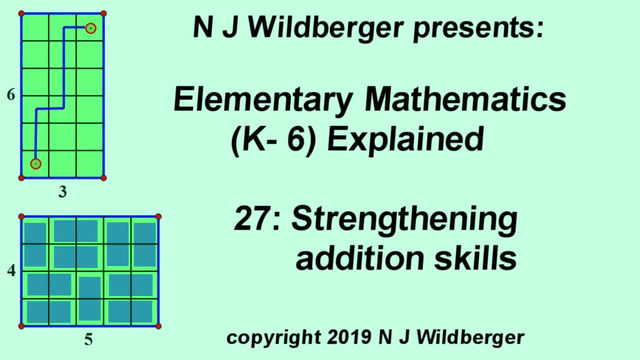 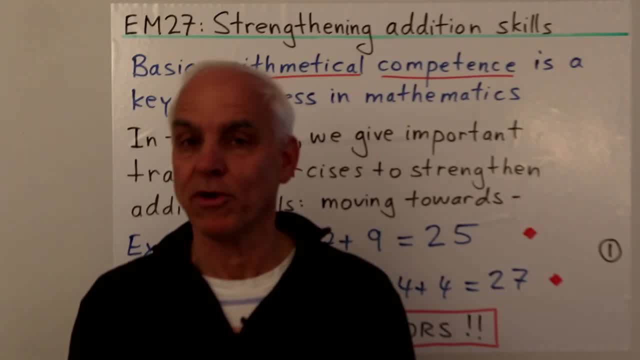 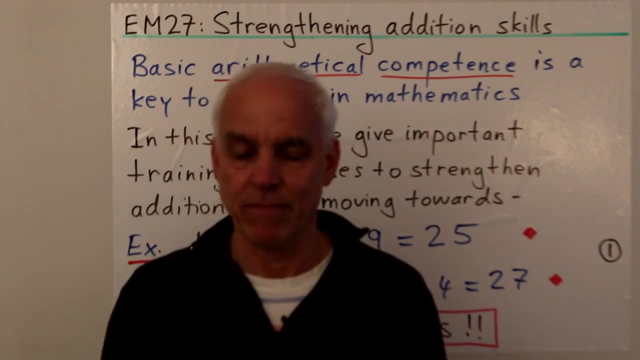 Welcome everyone, I'm Norman Welberger. In today's video we are going to strengthen addition skills for young people, A very important, very important activity. that's really sort of a fundamental basis for success in mathematics. Okay, so what we're doing is we're. 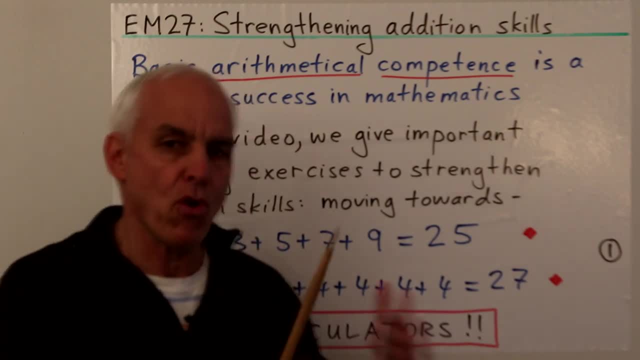 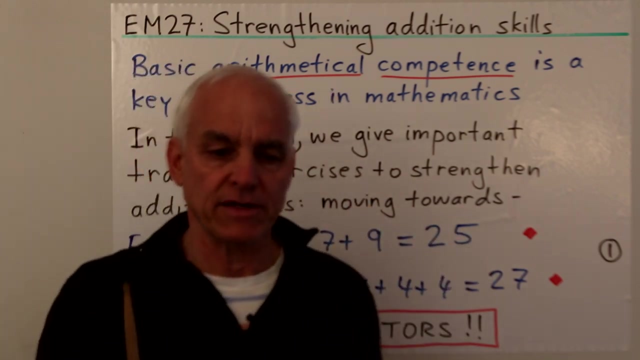 going to lay out a way of thinking kind of a program of proceeding in small stages, starting from very simple fundamental concepts and techniques to higher ones. So there will be a kind of an evolution of techniques that we'll develop. There'll be some novel ideas and maybe 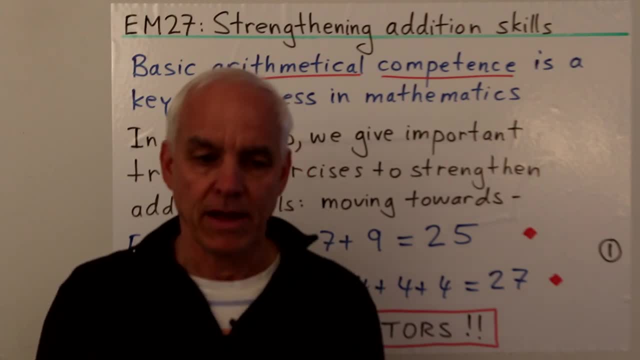 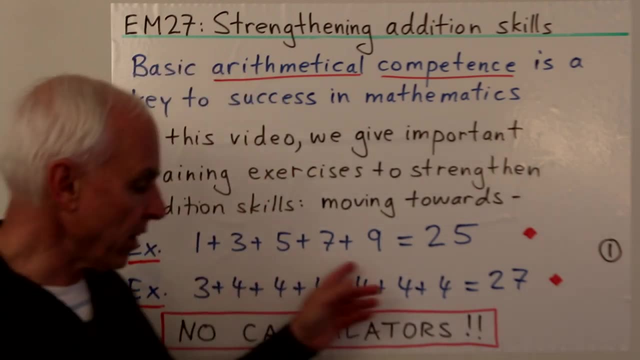 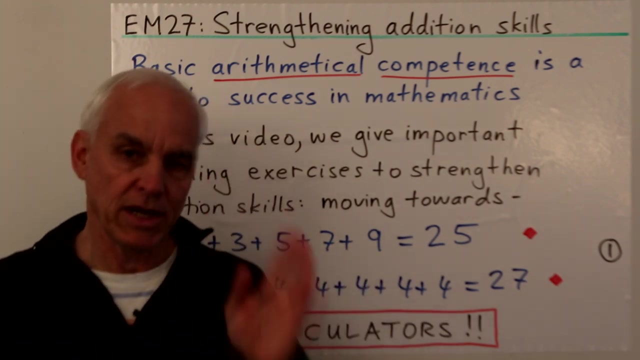 even some notions that you have not run across before, but I think they will be important in strengthening our students' arithmetic medical skills. What we're aiming for ultimately is something like this: that when a student sees 1 plus 3 plus 5 plus 7 plus 9, here's what they do- They do it in their heads. okay, They say: 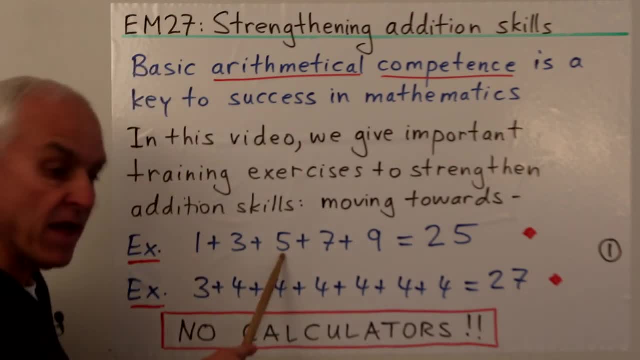 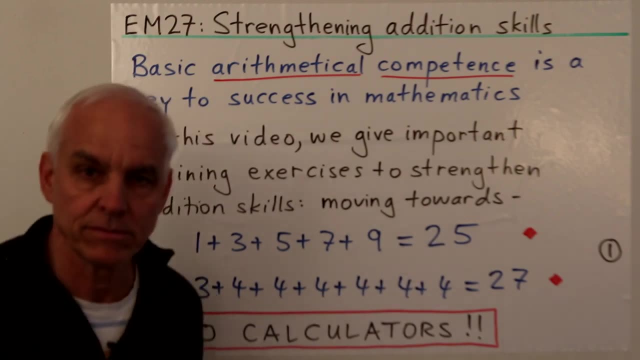 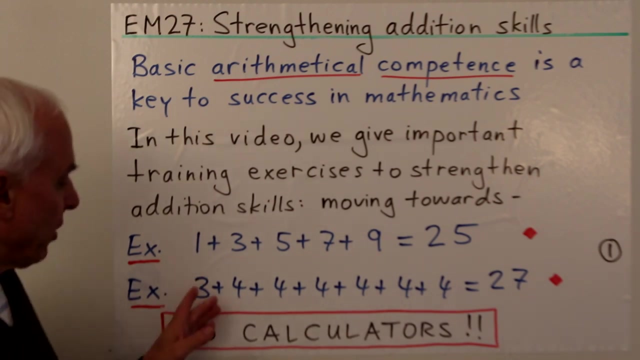 okay, 1 plus 3 is 4.. Add 5,, that's 9.. Add 7, that's 16.. Add 9, that's 25.. Another kind of example that we'll be looking at more extensively in a later video is this kind of thing where you. 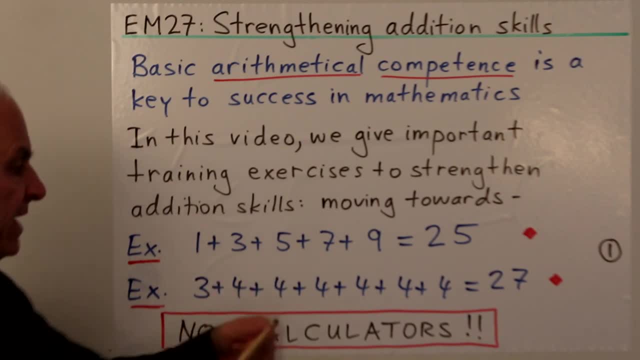 have essentially an arithmetical sequence built up by adding the same quantity. That's actually quite important. So here to add up this 3 with all these 4s: 3 plus 4 is 7 plus 4 is 11 plus 4 is: 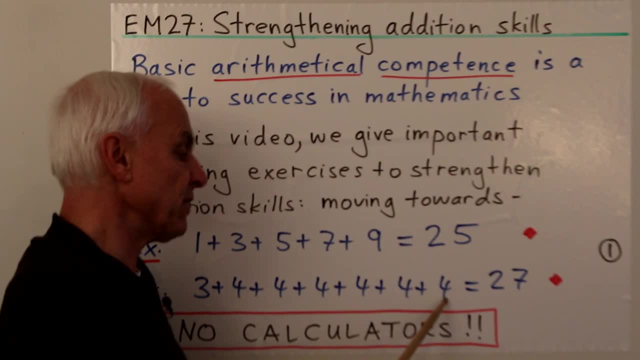 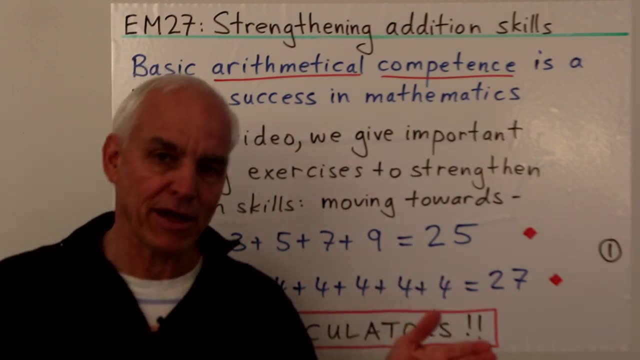 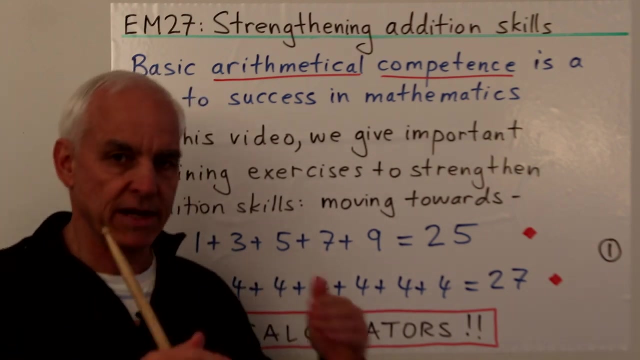 15 plus 4 is 19, plus 4 is 23, plus 4 is 27.. So that kind of facility to be able to do that smoothly, accurately, confidently is so important, Aiming then towards establishing the techniques that allow young people to develop those crucially 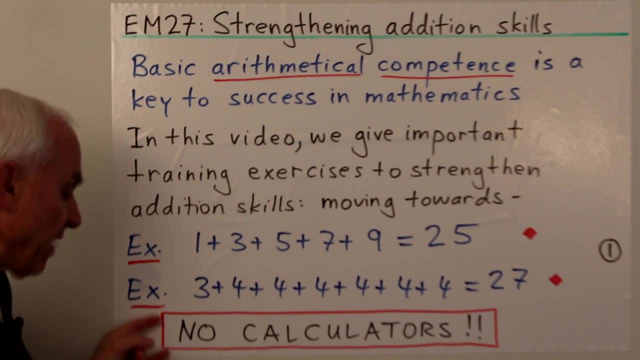 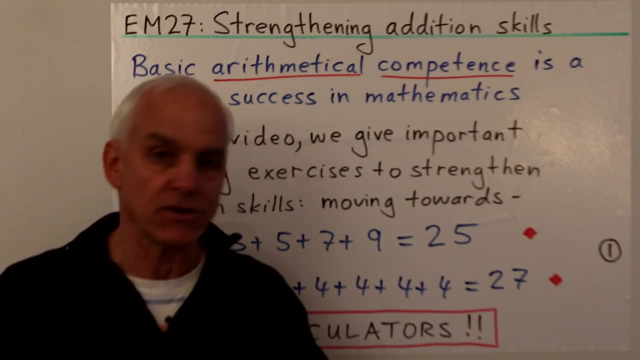 important skills. Now I want to emphasize very, very strongly, okay, that calculators are not part of this picture at all, Not at all. So, as far as I'm concerned, K to 6 students should not even know what a calculator is. They should not have ever seen one. okay, If there's one around, put it away. 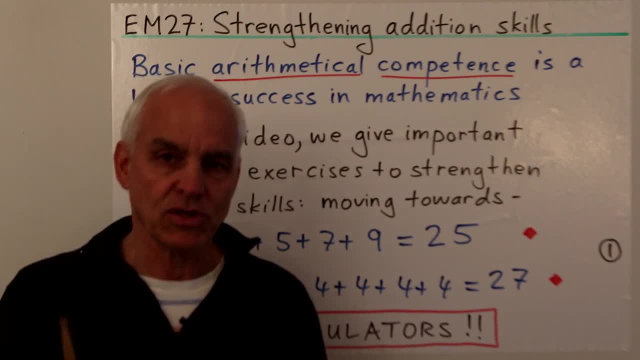 lock it up behind you. Okay, If there's one around, put it away. lock it up behind you. If there's one around, put it away. lock it up behind you. Lock and key. Do not let the students rely on calculators. I know there are trends in modern. 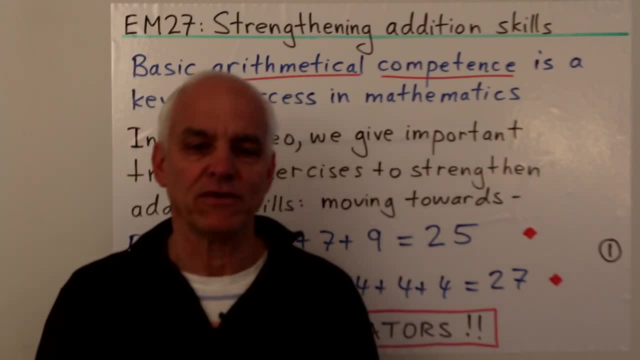 education circles, to you know, to use technology effectively and to introduce young children to calculators and computers at an early age. I think there is role for computers but not calculators. Okay, The actual arithmetical computations have to be done by the student. In fact, we are going to 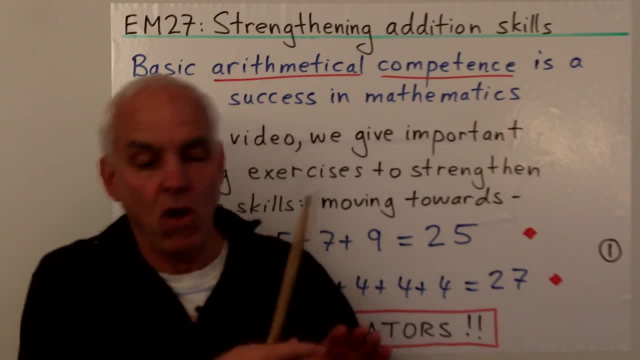 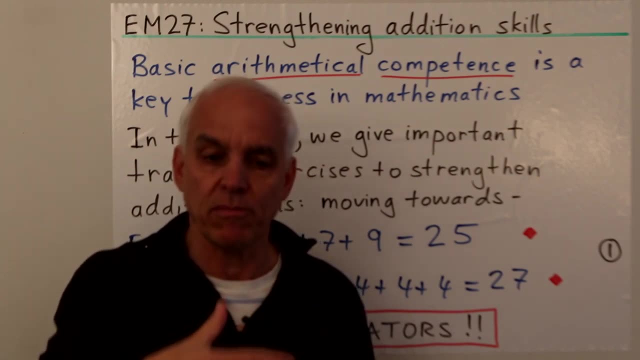 start by getting them to do these things mentally. Later on, when the numbers get bigger, they'll have to augment their mental skills with actual writing. Okay, That'll also be important, But at this stage we're talking about adding relatively simple numbers, typically natural numbers less than 10. 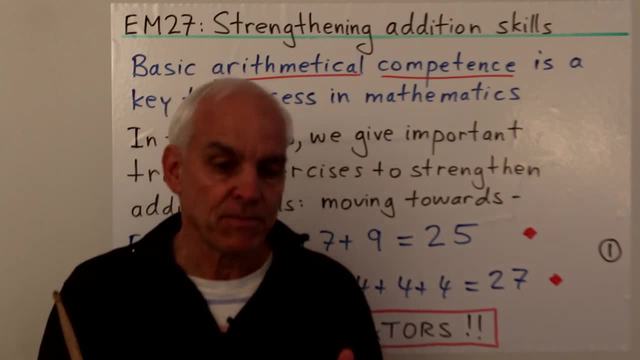 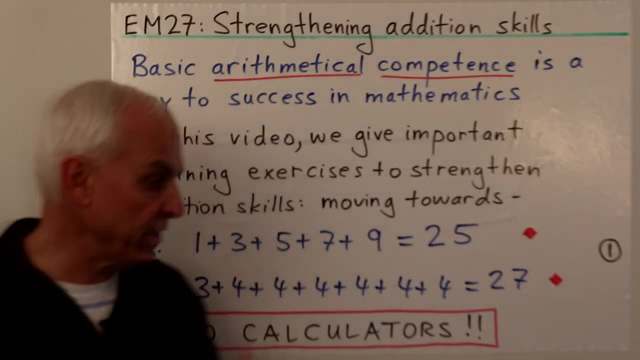 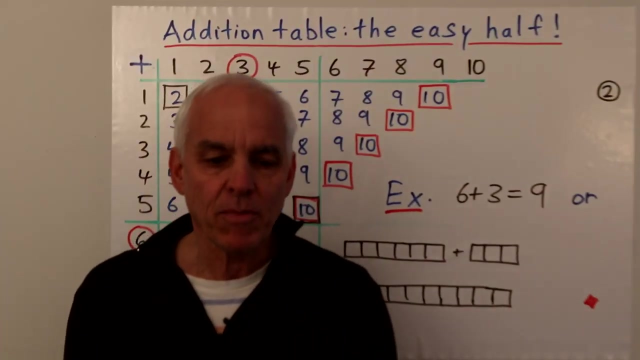 to themselves perhaps a number of times, And for that we can do it in our heads. The young children should be able to learn how to do that. That's what we're aiming for. Okay, so please emphasis, no calculators at all in this story. Now we've already seen the addition table We're going to have. 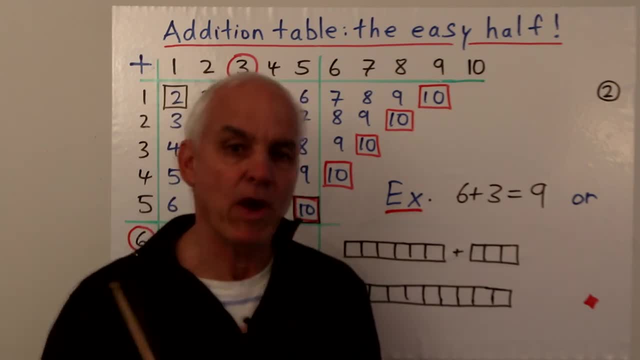 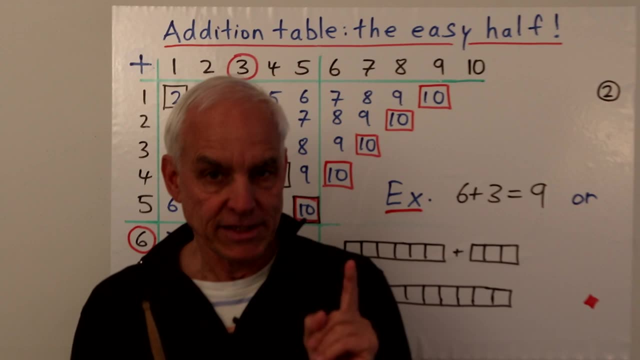 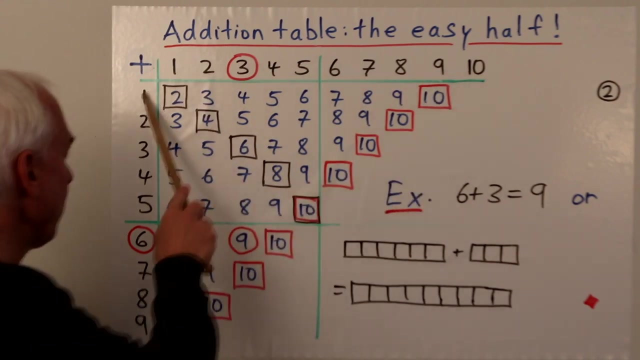 another look at it today, but in sort of two halves. There's a kind of easy half to the addition table and there's a harder half. It makes sense to start with the easy half. Here is the easy half of the addition table, Numbers 1 to 10, numbers 1 to 10.. The entries here represent the sum of the. 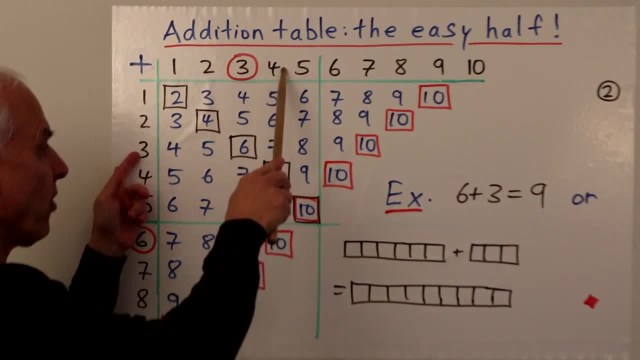 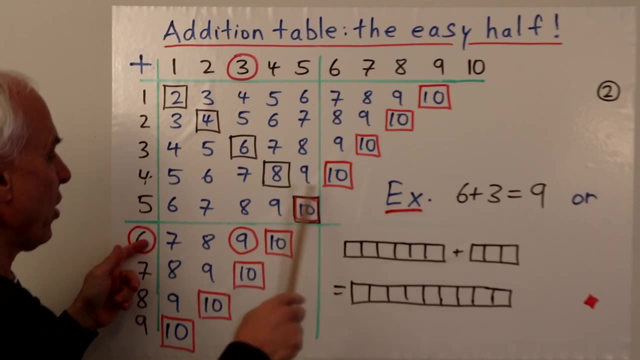 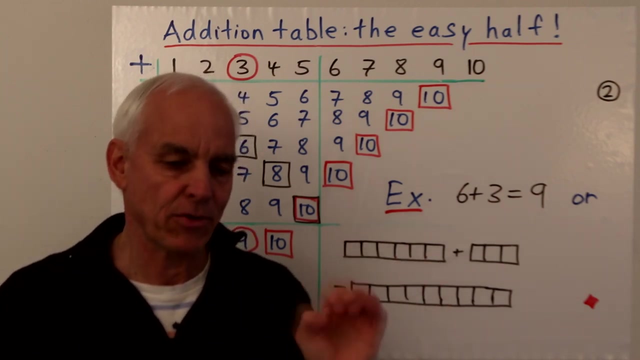 numbers in the left-hand column And in the top row. So 3 plus 4 is 7.. 4 plus 5 is 9.. 6 plus 3, circled here, is 9.. And these are the results, where the end result is a number less than or equal to 10.. Okay, less than or equal to 10.. 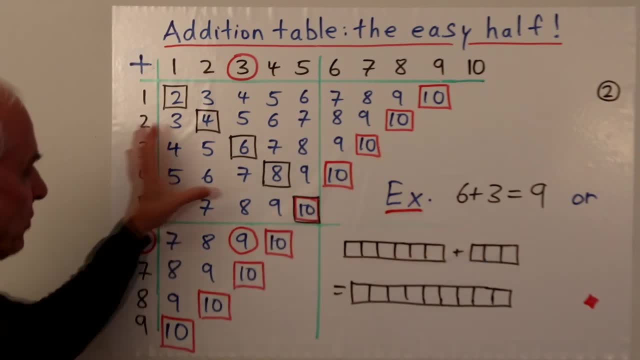 So we've ignored all the other ones. Now what we want to do is we want to get students just familiar with the numbers. So we want to get them familiar with the numbers And we want to get familiar with the numbers. And we want to get them familiar with the numbers And we want to get 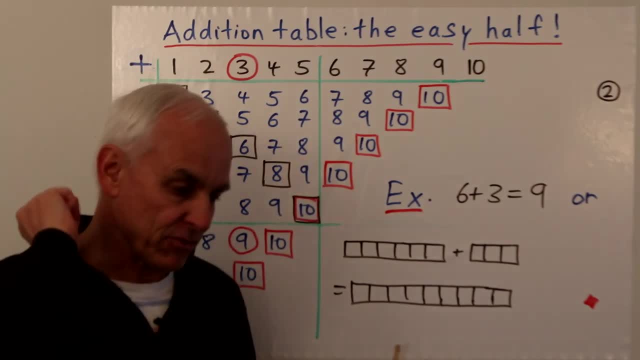 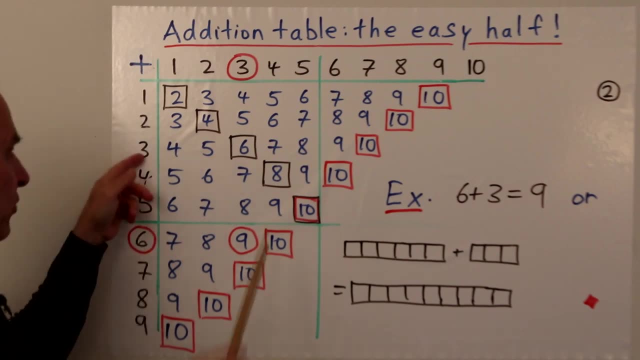 them familiar with this half of the addition table, so that it becomes rock solid, so that they immediately know that 4 plus 5 is 9,, that 2 plus 7 is 9,, that 3 plus 5 is 8, etc. And I remind you. 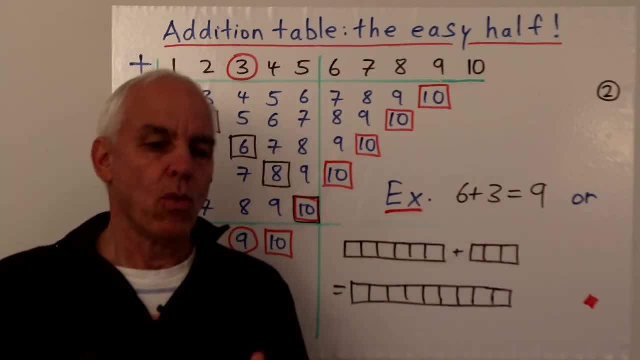 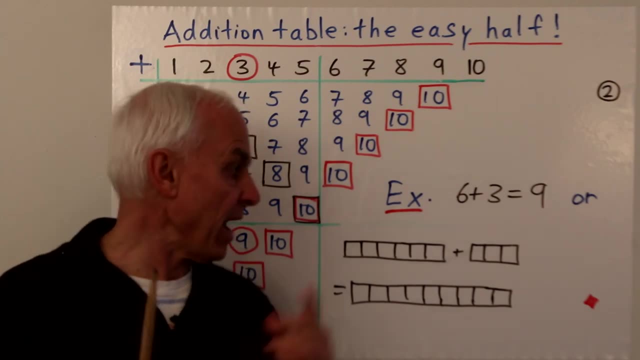 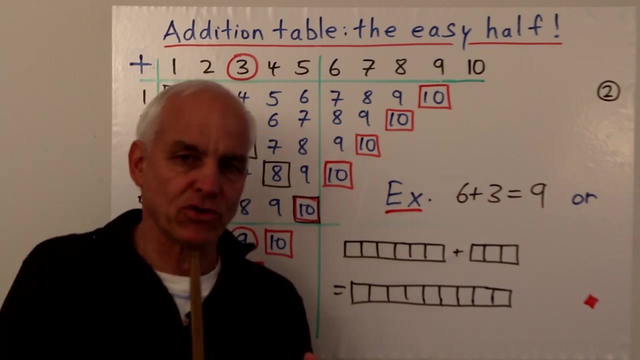 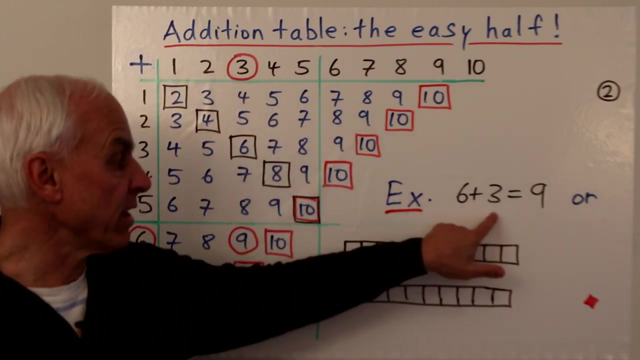 that when we're doing very simple addition like this, we can visualize what's going on in terms of our fundamental interpretation of natural numbers as row rectangles. Okay, that was what I suggested was a natural, very geometrical, physical representation of what a natural number actually is. so when we add six plus three, what we're doing is: 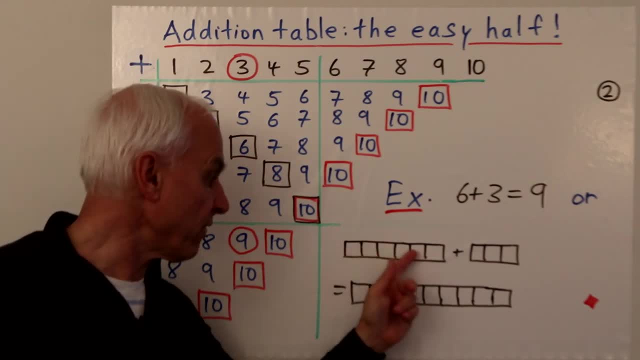 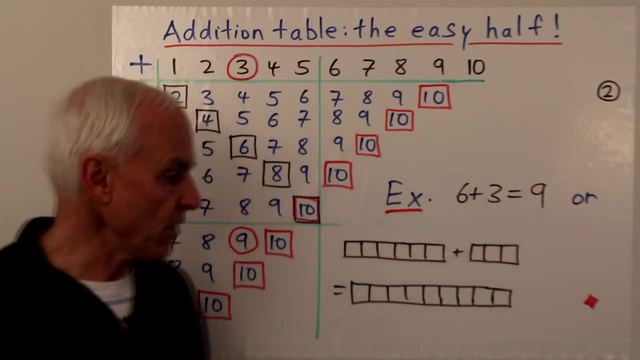 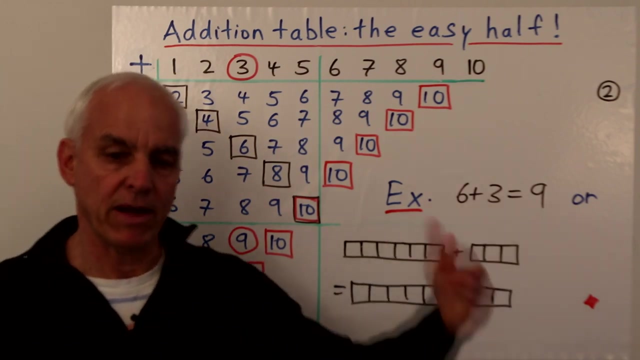 we're taking this row rectangle with one, two, three, four, five, six boxes and this one with three boxes and adding them together and that's a physical process resulting in a rectangle with nine boxes. so this is the geometrical interpretation of this arithmetical thing that we want to keep in mind all. 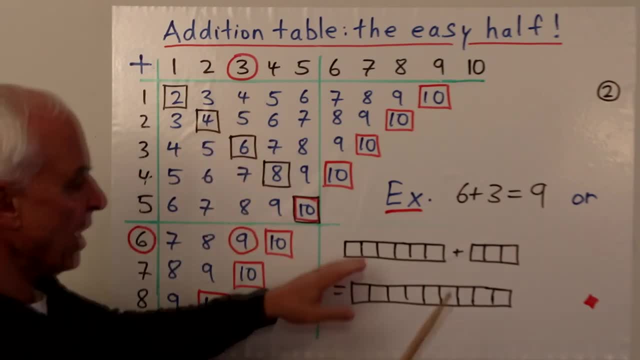 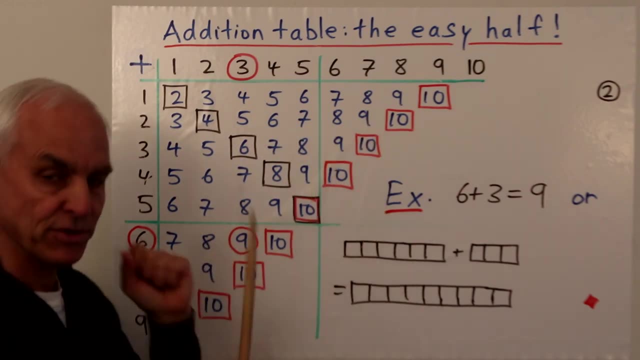 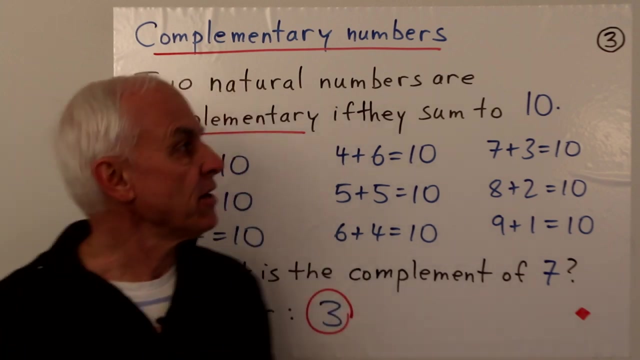 right. so behind each one of these additions, there's our little diagram like this, that tells you what happens if you have a certain number of boxes and another certain number of boxes and you put those two boxes together. now let's introduce a useful terminology, the idea of complementary numbers. now this has to. 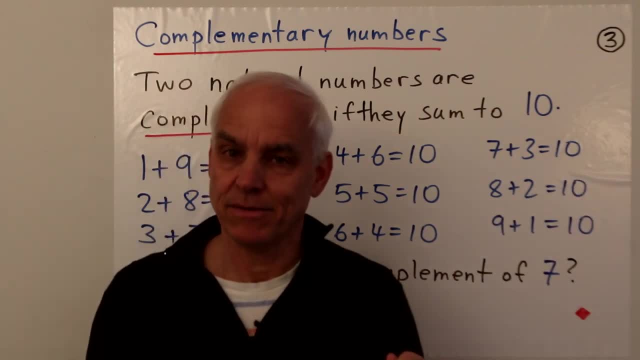 do with the numbers on the table that add up to ten. you're not going to be able to remember all the numbers. you're going to have to remember all the numbers you're going to have. previous slide: I put those in red. That's a particularly kind of important situation when 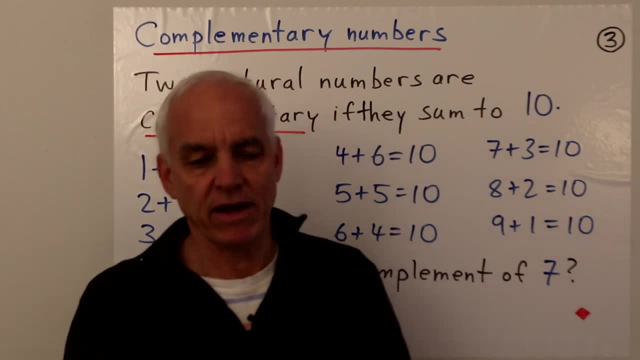 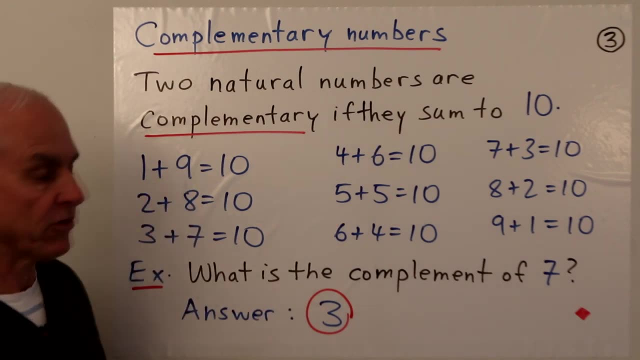 you have two numbers adding up to 10. And so we give that a name. We say that they're complementary numbers. Two natural numbers are complementary if they sum to 10.. So, for example, 1 and 9 are complementary, because 1 plus 9 is 10.. 2 and 8 are complementary. 3 and 7 are complementary. 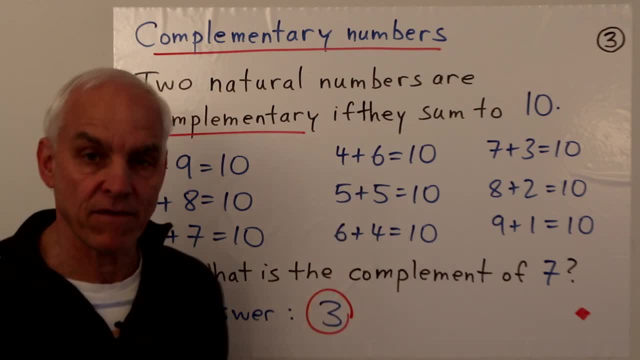 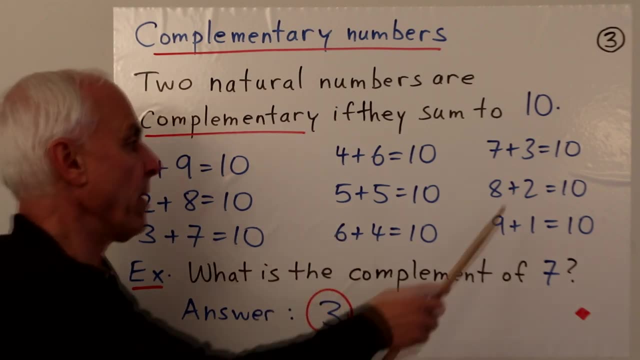 4 and 6 are complementary And 5 and 5 are complementary. So 5 is complementary to itself. But we can also do it in the other way, So we can say 6 and 4 are complementary, Or 7 and 3. 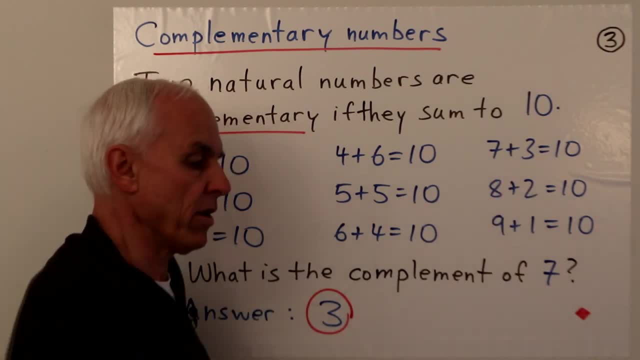 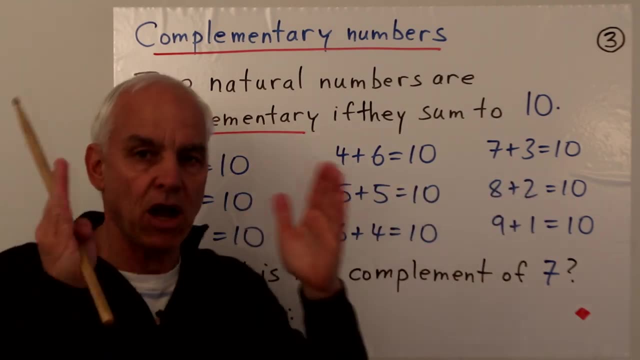 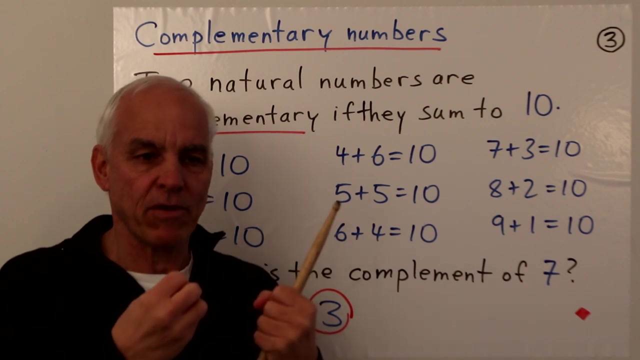 are complementary, Or 8 and 2 are complementary, Or 9 and 1 are complementary. So the young child should learn all of these So that 8 and 2, ah, those are complementary numbers. There's something that twigs when they see 8 and 2 together. Those two numbers have a particularly important. 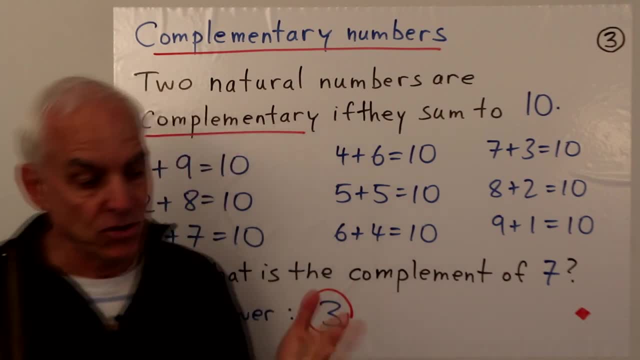 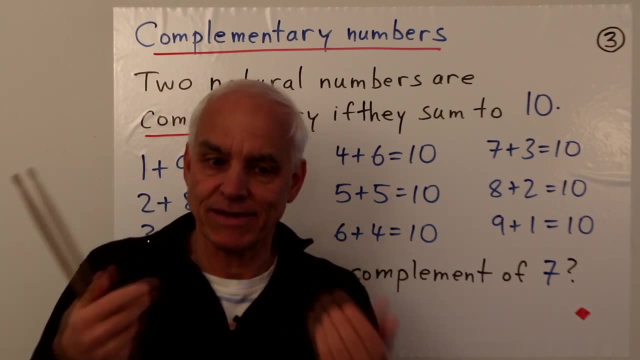 relationship. Now we should say that this is because of the all-importance of our data. So we should say that this is because of the all-importance of our data, Decimal number system, right, the fact that we're using the Hindu Arabic system, which relies on 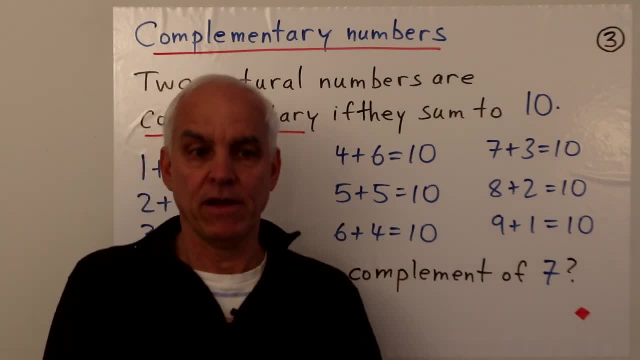 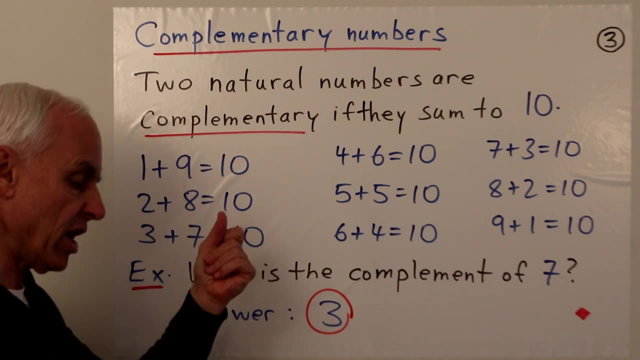 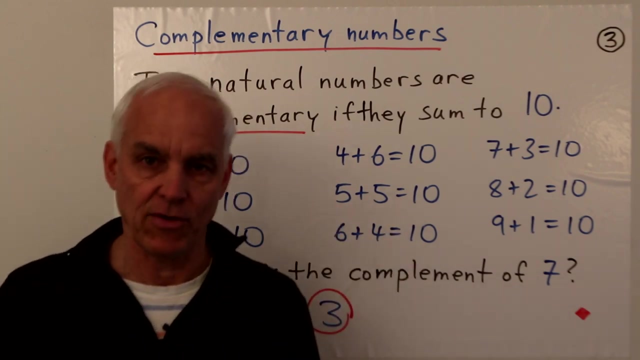 Powers of ten. that's why this notion is so important for our arithmetic. So we have very simple but fundamental questions like: what is the complement of seven? the child should immediately know that it's three. Okay, no thought required. complement of five: It's five. complement of four: It's six, etc. 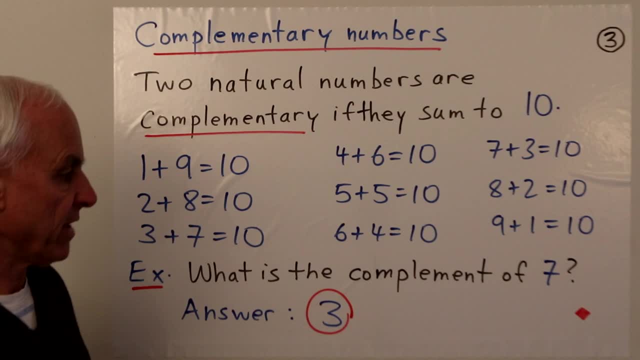 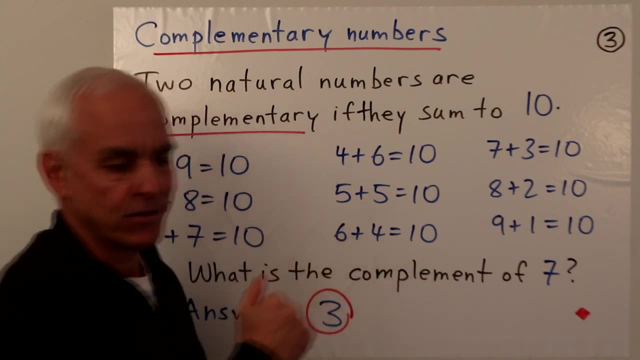 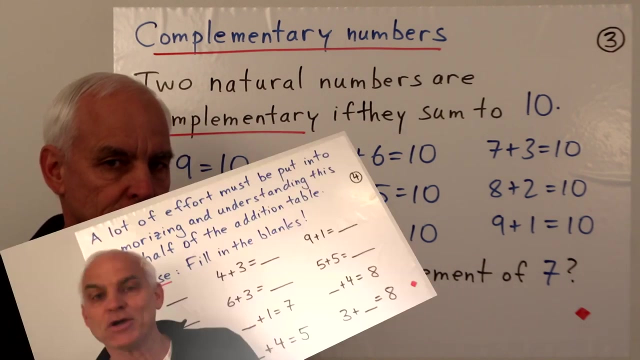 okay, so drill that into them. and Geometrically that means that we're taking the two boxes that represent the two numbers, putting them together and we get Total sum of ten. that's sort of like a standard unit, an important unit for four numbers. So a lot of effort must be put in to 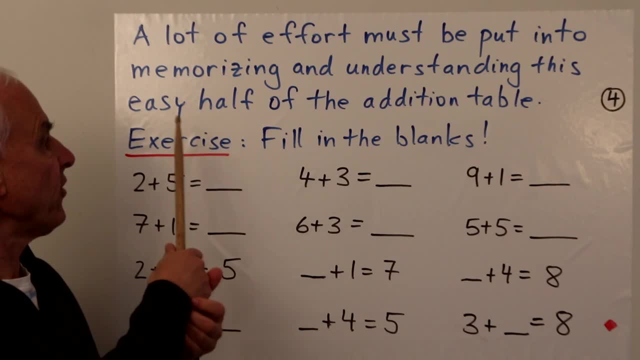 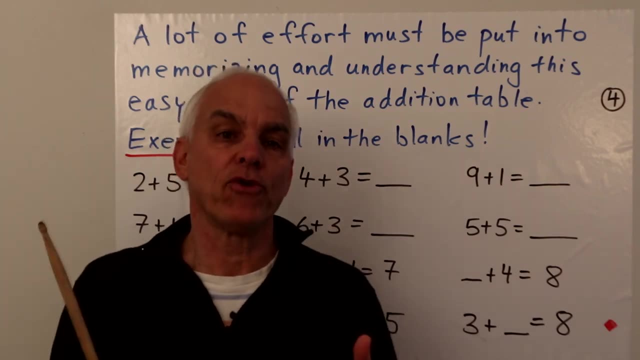 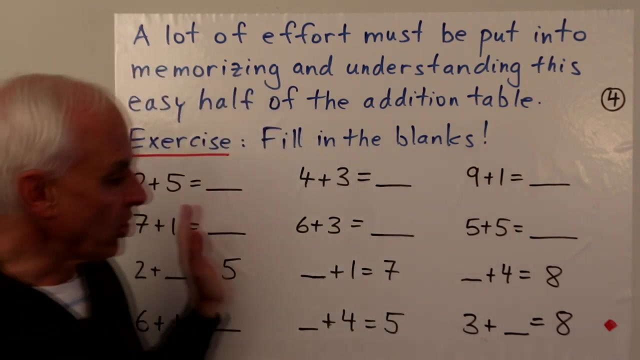 memorizing and understanding Geometrically this easy half of the addition table. So when we have two natural numbers Less than ten whose sum is also less than or equal to ten, Okay, so now we can give students lots and lots of questions to practice. Okay, so they become familiar. 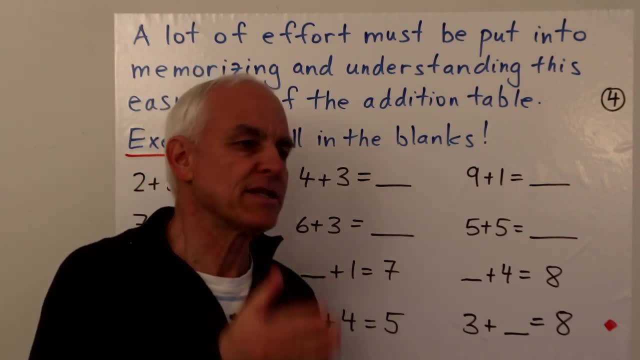 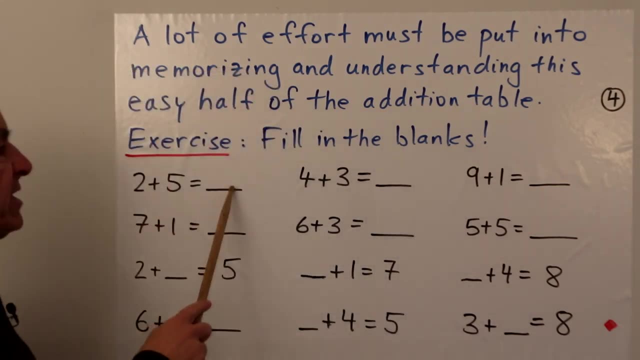 with these things, and so they're able to Do these kinds of simple additions Automatically without any thought at all. They just boom. the answer is right there. two plus five is seven. four plus three is seven. nine plus one is ten. seven plus one is eight. Six plus three is nine. five plus five is ten. two plus something is five. That's a little bit trickier. 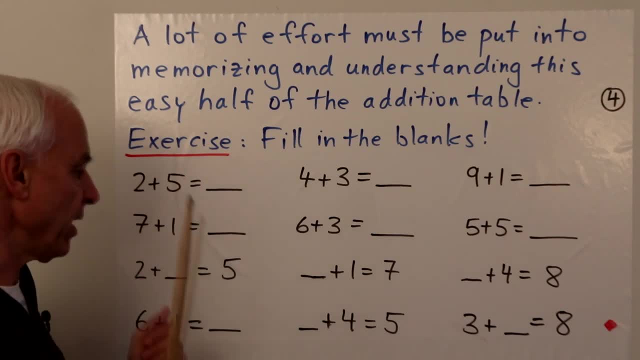 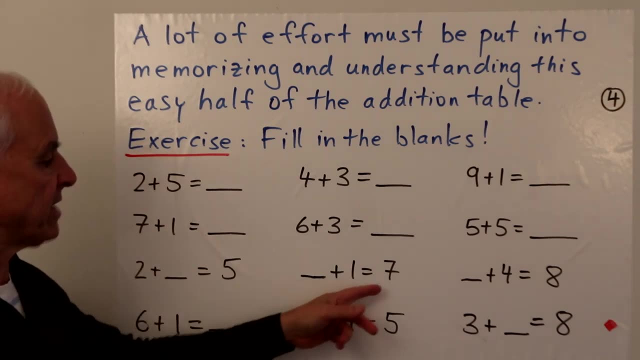 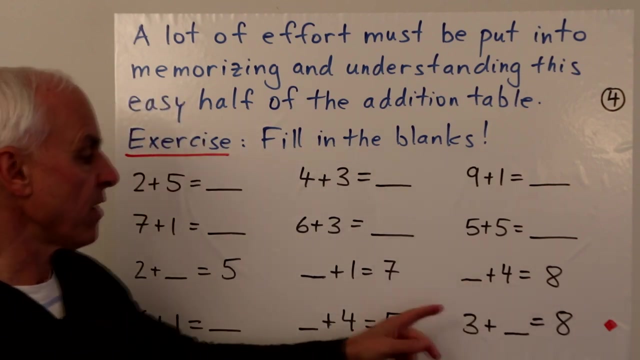 Okay. so we still have to understand the story, but from a slightly different point of view. two plus three is five. Okay, two plus three is something plus one is seven. six plus one is seven. Four plus four is eight. six plus one is seven. one plus four is five. three plus five is eight. 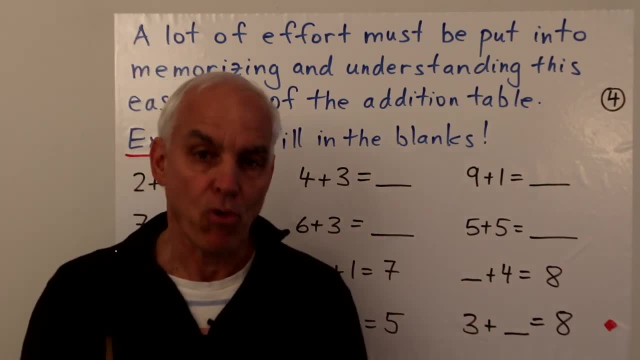 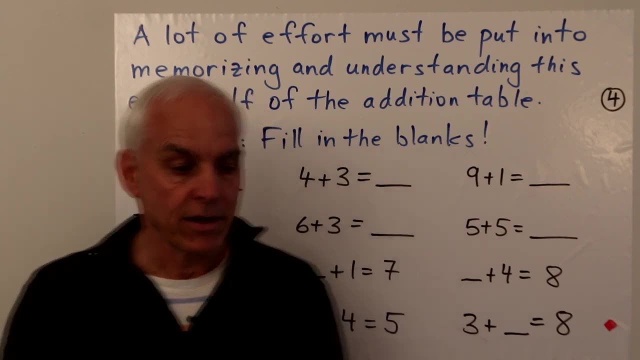 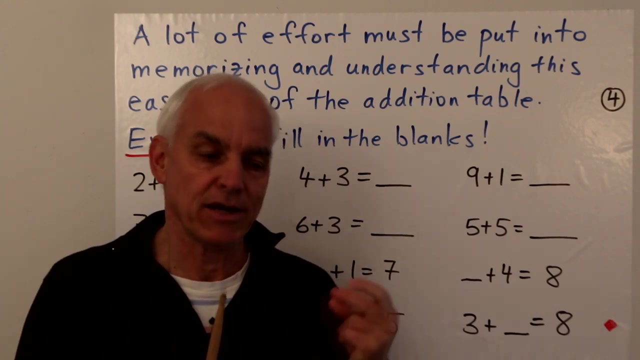 Now, hopefully, you can all do these things in your sleep, but it's important to get your child to be able to do these things in their sleep as well, and for this, You know, a program of practice and training has to be put into place. It's not something that they just learn. 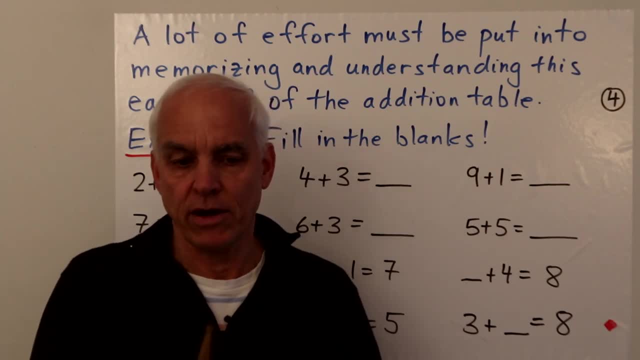 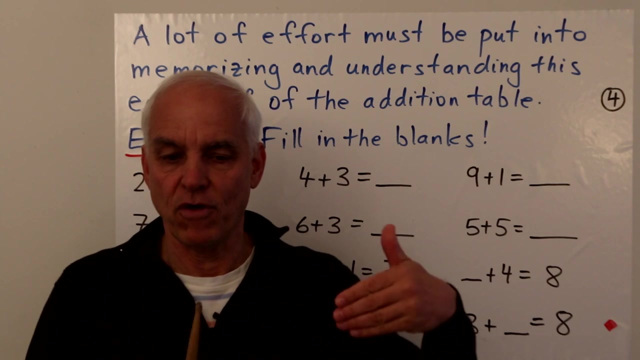 immediately from one day to another. and Here's where educators have to have to step up and sort of enunciate Programs of training. how do we train young children? What are the natural steps so that they become familiar with this? This half of the addition table. 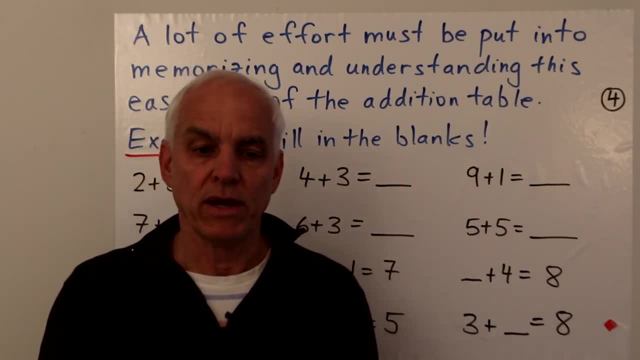 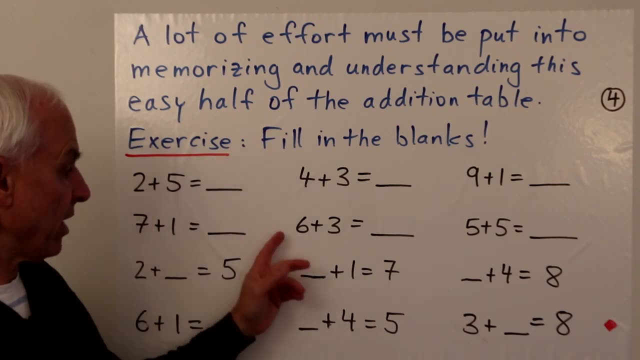 Okay, but in any case, they should be doing many, many problems Just like this, and in fact, this is actually quite a good format. I think we have two Numbers like this and there's a blank somewhere, and they actually have to fill in the blank. 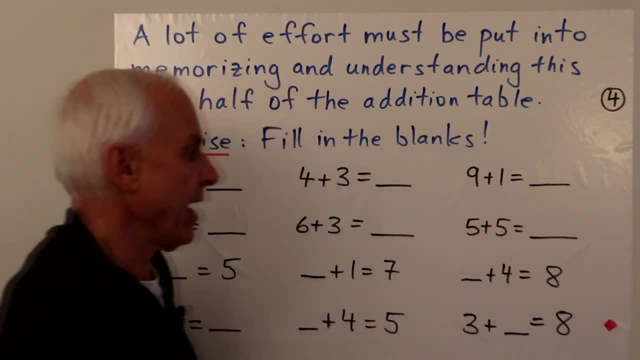 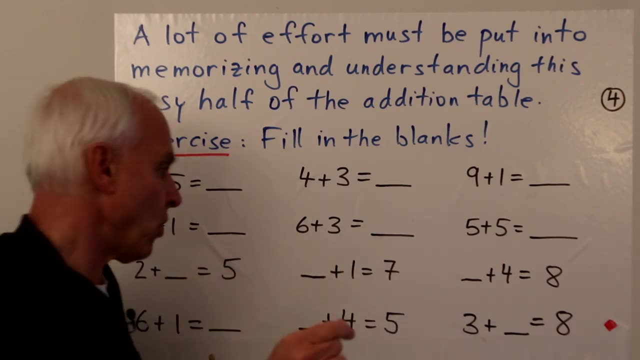 okay, so they have to write something and- And They don't have to do much else- game. We're not asking them to to rewrite the entire equation, we just want the answer and we want them to write it down. it has to be legible and correct and 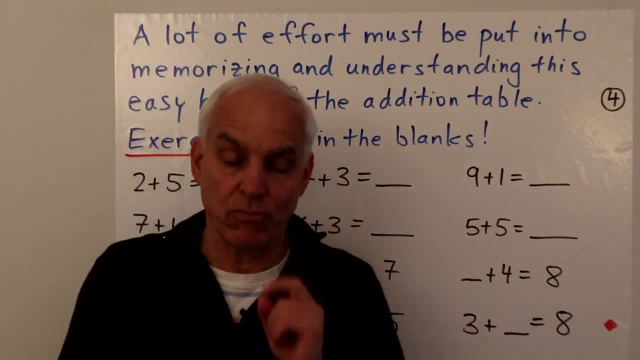 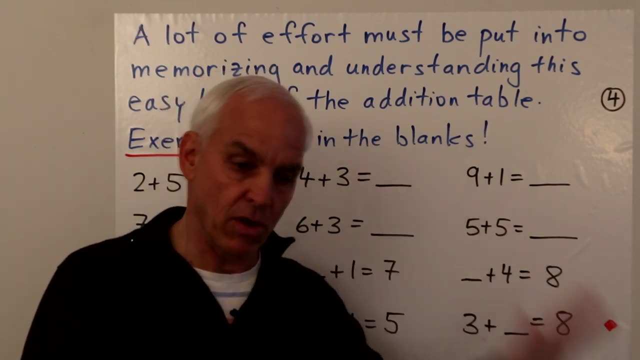 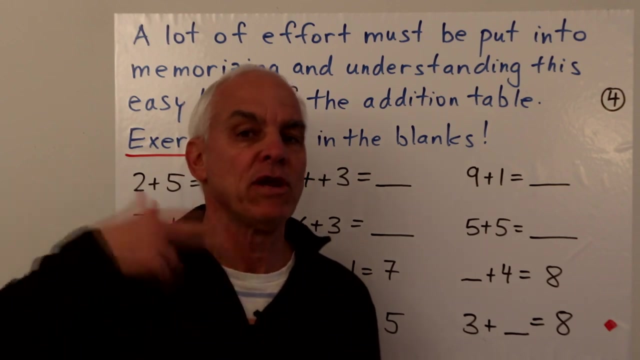 Literally, you can give them hundreds of problems like this, and probably they should be given hundreds of problems, Maybe even thousands. Okay, it doesn't take long. once they're good at this, They can do a lot very quickly, And so we have to do so many that they're they're really good at this, and then we have to reinforce this. 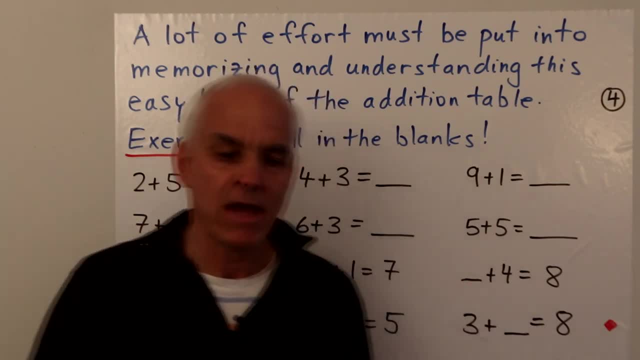 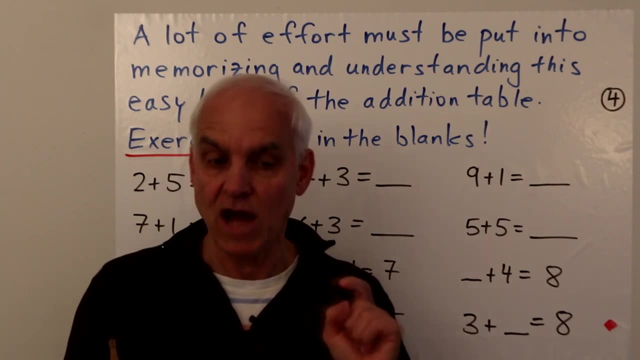 So, as the years go by- maybe this is the very early years- as the years go by, We need to come back and revisit this kind of fundamental skill. Okay, so it's not just a skill for year one students, It's also a skill for higher year students. 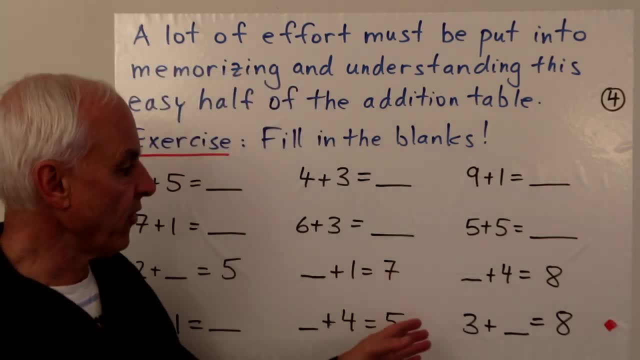 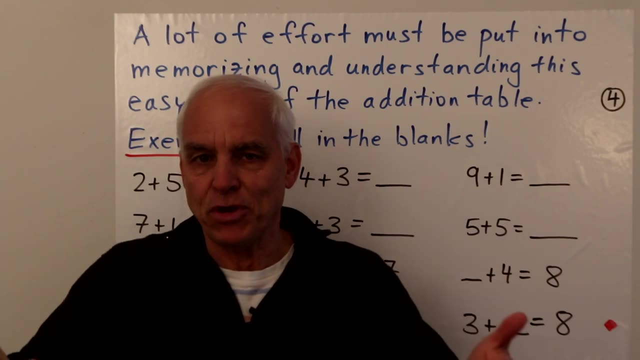 But of course, you can give them a little bit more sophisticated problems, and I'll show you a few of those- Those later on, Okay. but so I want to emphasize that, even though this video that I'm showing you now is relatively short video, still the amount of training and and 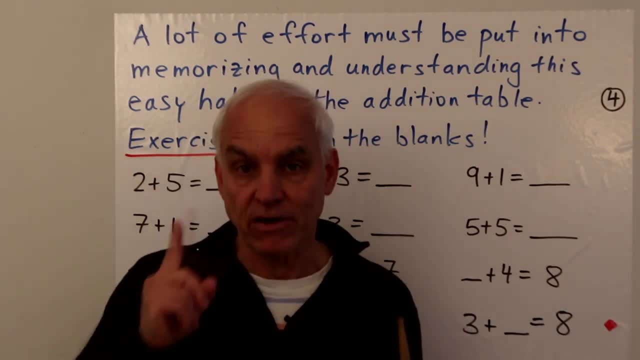 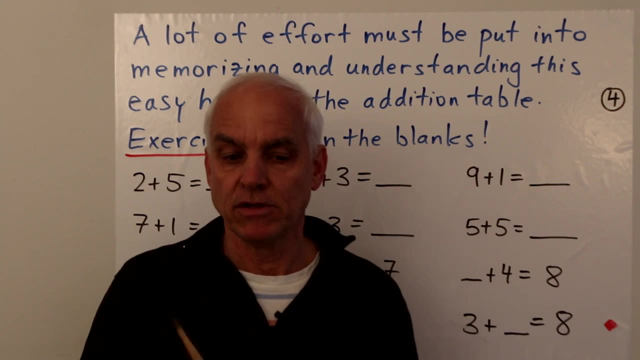 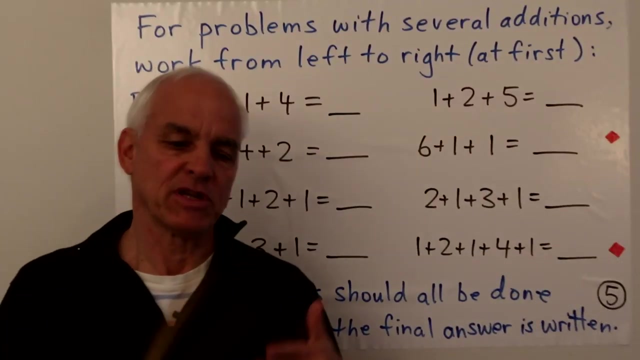 practice required to absorb this material Is very substantial. we're talking weeks, perhaps months, of Training for young people to ingest everything that's happening here, to become really fluid with the computations. So after some time a student gained some confidence and competence. so we can go a little bit further. 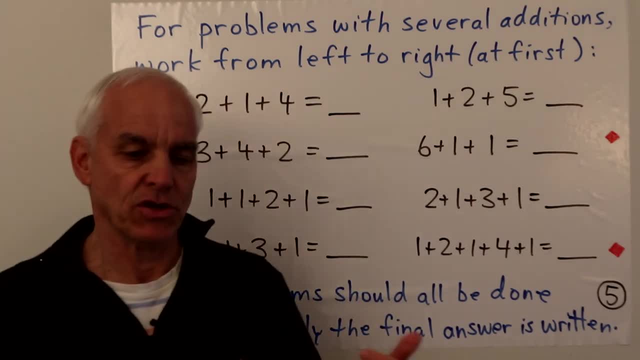 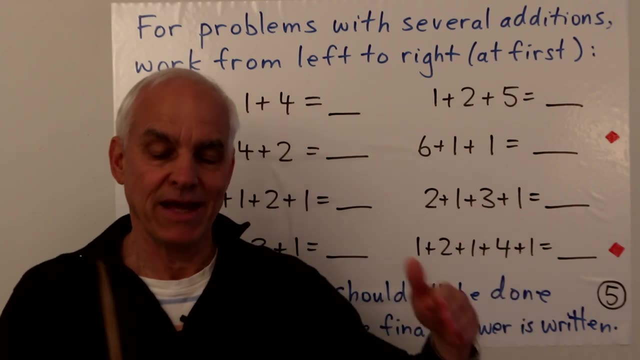 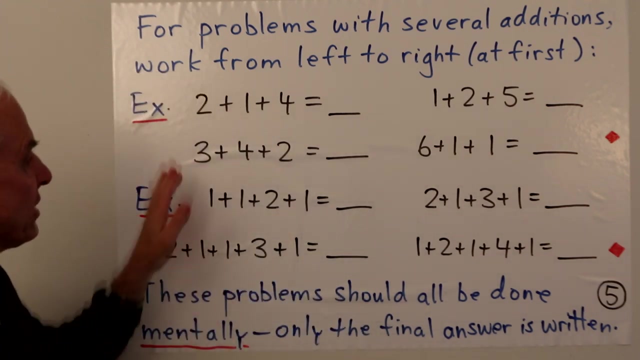 We can give them problems that involve several additions all at once, But these are still relatively easy in that the total sums that we get are still less than or equal to ten. So we're still always relying on that easier half of the addition table and I suggest that these problems are done from left to right, so the students just automatically goes from left to right. 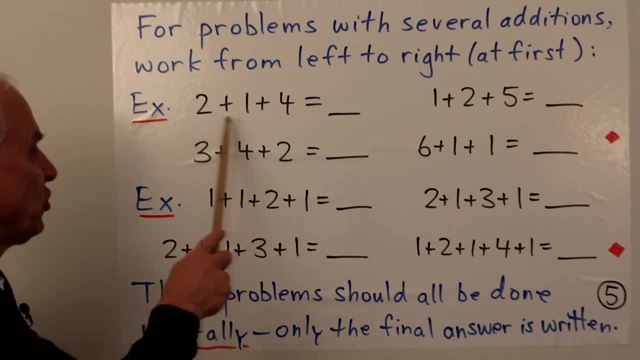 So let me illustrate what they should be doing. So we need to add up two plus one plus four. start from the left: two plus one is three. We just record that mentally- three, and now we have to add four. So it's three plus four, which is seven. 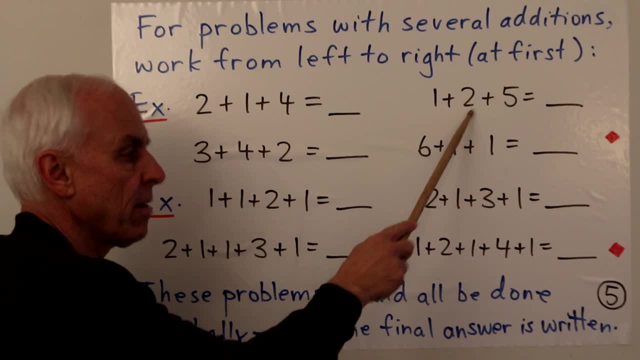 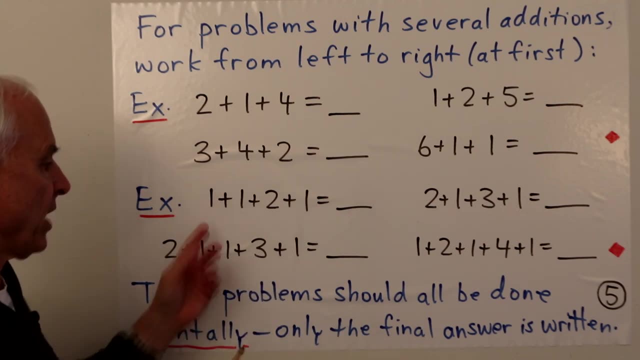 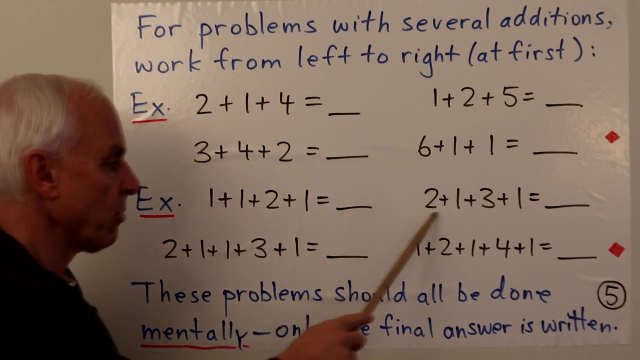 one plus two plus five. One plus two is three plus five is eight. Three plus four is seven plus two is nine, etc. You have more than three. one plus one is two plus two is four plus one is five. Two plus one is three plus three is six plus one is seven. 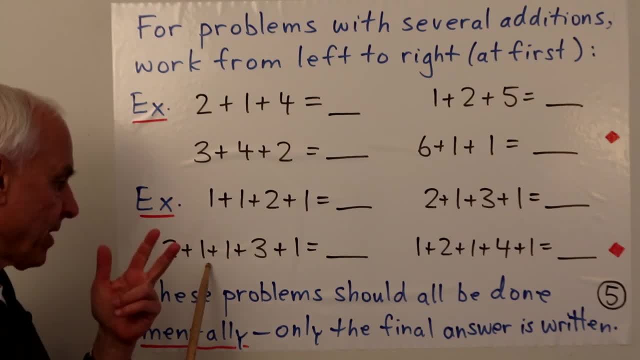 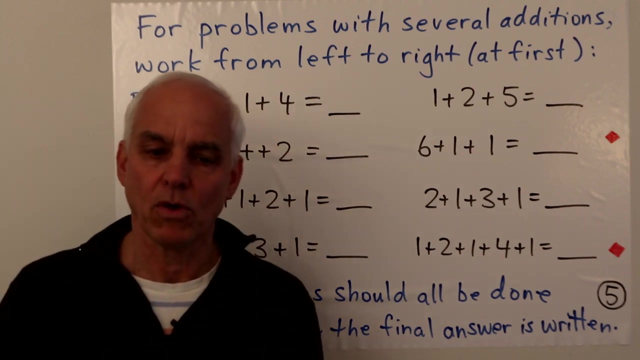 So note the way I'm saying it: two plus one is three, plus one is four, plus three is seven, plus one is eight. Okay, so kind of efficient mental way of going through it. So these problems should all be done mentally. We're just relying on our mental. 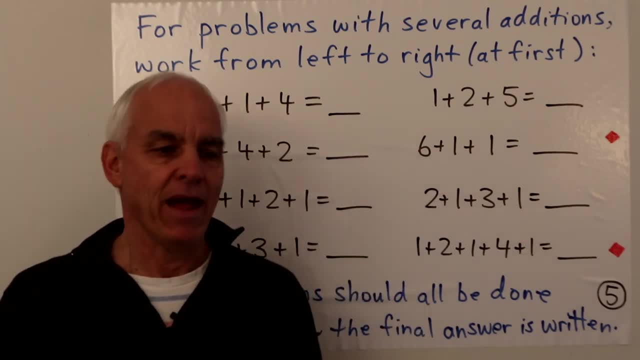 recall of the addition table, the easy half, and then subsequently Performing more and more additions, always relying on that fundamental understanding that hopefully we have. So the only thing the students actually writing down is the final answer. Okay, none of the intermediate steps. Now we've talked about two numbers being complements of each other when they add up to ten. 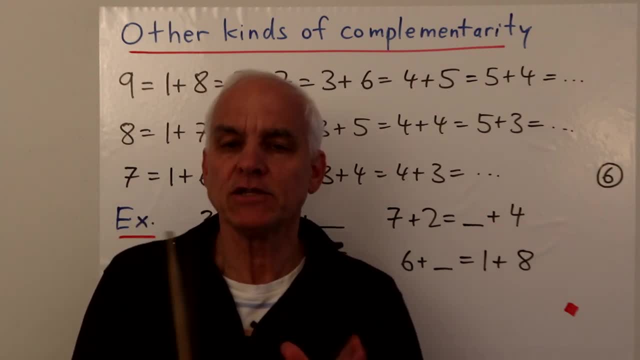 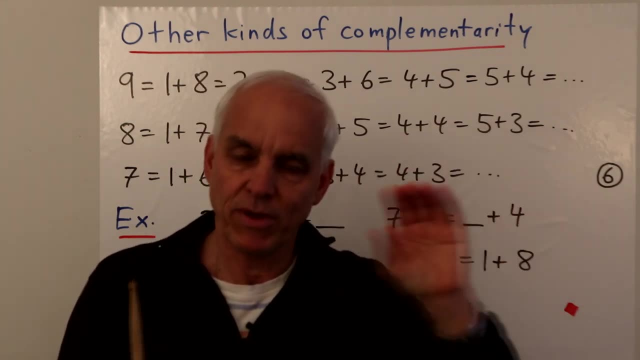 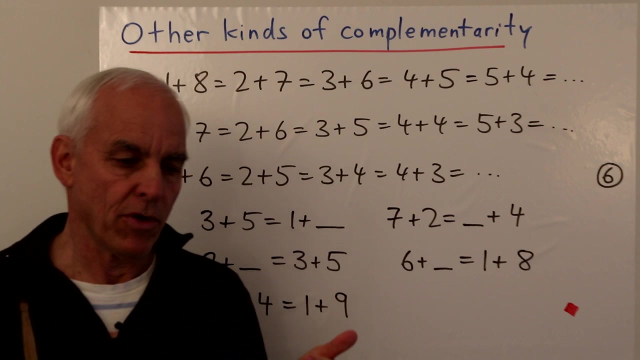 but there are other versions of that Kinds of complementarity that are also useful for the students to know, Associated not with the number ten but with other lesser numbers. so, for example, nine Nine can be written as a sum of two natural numbers in a number of ways, and 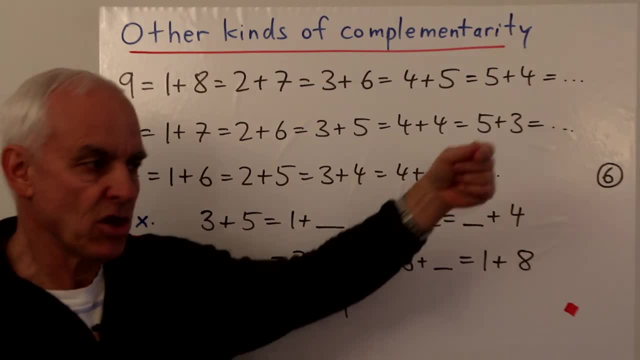 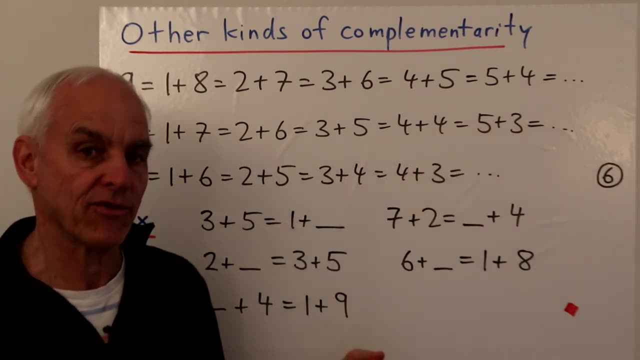 You can see that quite easily. if you go back to the addition table, You just go down the diagonal that's going this way. There's a diagonal of tens and this. just right above it There's a diagonal of nines that illustrates all the pairs that sum to nine. 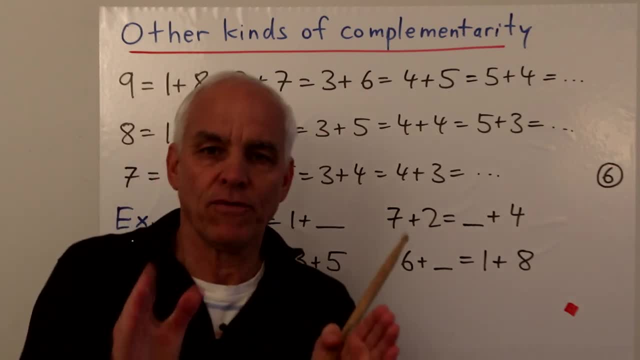 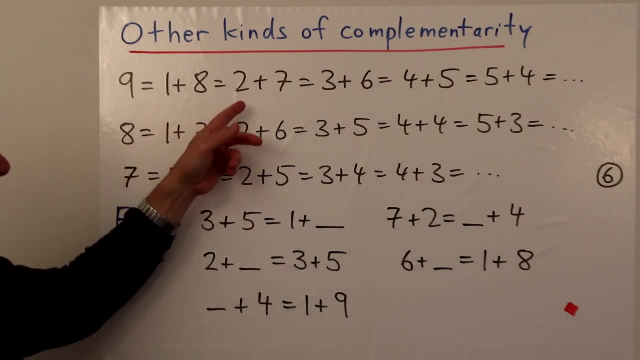 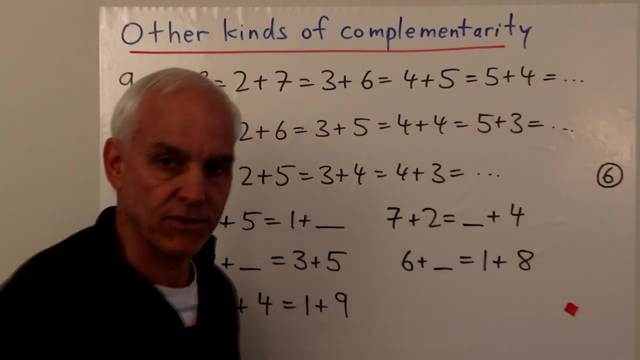 so it's useful for Students to see all of those pairs at the same time to be able to compare them. Okay, so here I've given: one plus eight equals two plus seven, equals three plus six, equals four plus five equals five plus four, and you should actually complete this. 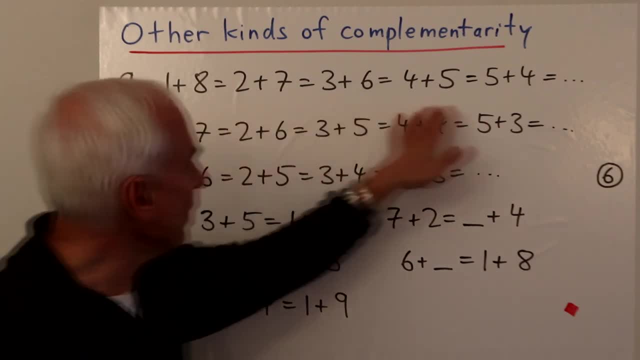 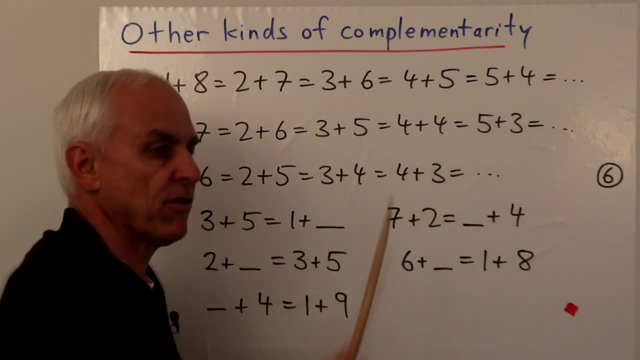 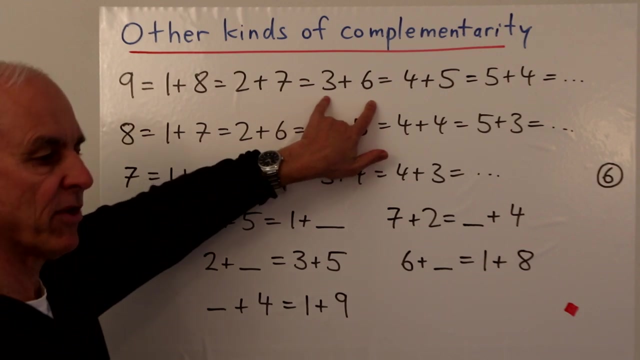 So you see all of them, Okay. So the student can look at all of these and get familiar with the idea that two plus seven is the same as three plus six, Or it's the same as five plus four. Maybe they can even think in terms of, well, to go from two plus seven to three plus six. we could do that. 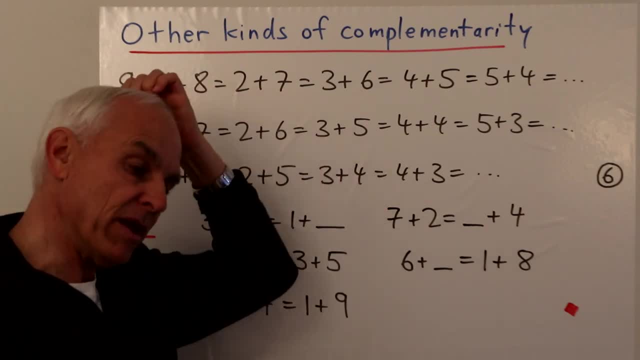 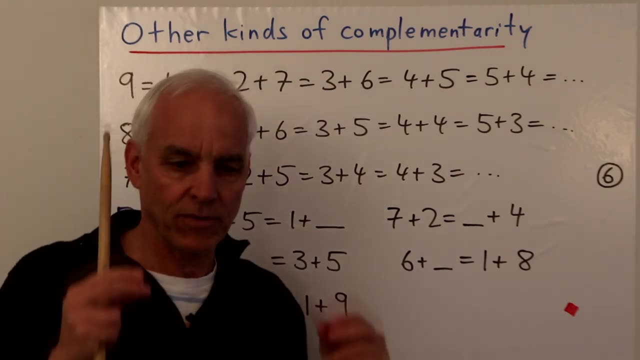 without actually evaluating the sum as being not, because the two has increased by one and The seven has decreased by one. So we've got two numbers. We're adding them together, We're increasing the first, Decreasing the second, so the sum is still the same. 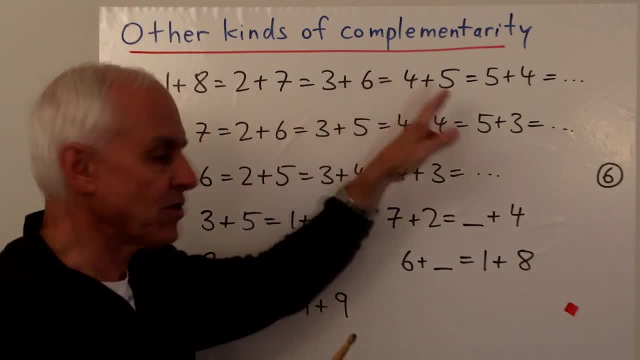 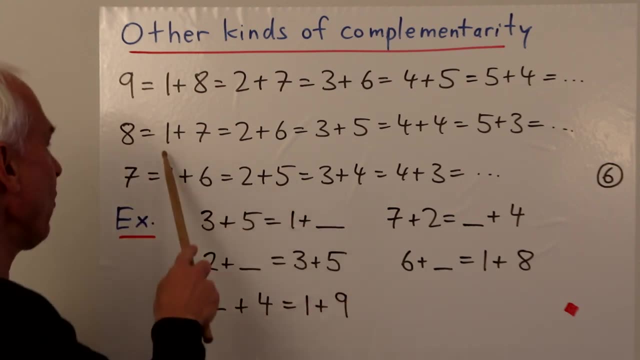 All right, that's sort of what's happening as we go from one of these to the next one. Here are the Complementary pairs for eight: eight is one plus seven, two plus six, three plus five, four plus four, five plus three, etc. And for seven, etc. 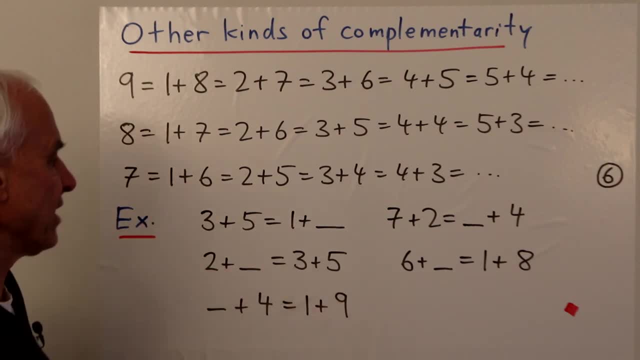 Okay, so now we can ask different kinds of questions, Such as: three plus five equals one plus what. There's a kind of a complementarity Problem, but having to do with eight, so three plus five is eight, What else do we have to add to one to get eight? 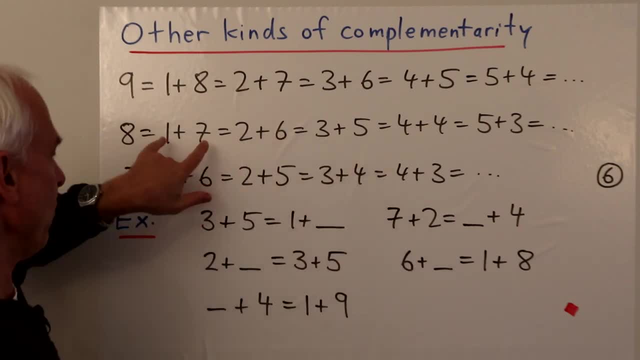 We're really taking the three plus five here and the one plus seven, and those are being used here Now. they don't have to memorize this exactly, but they just have to be familiar with it. They want, we want them to see these, these pairs, and become 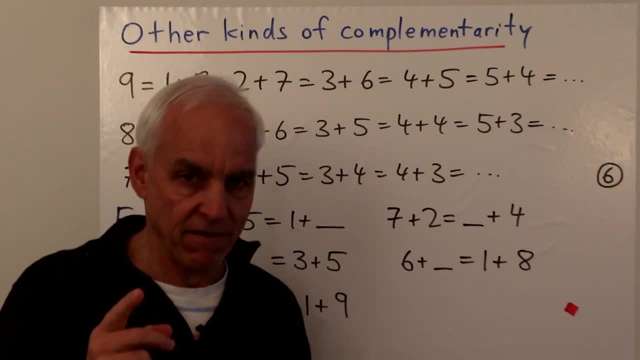 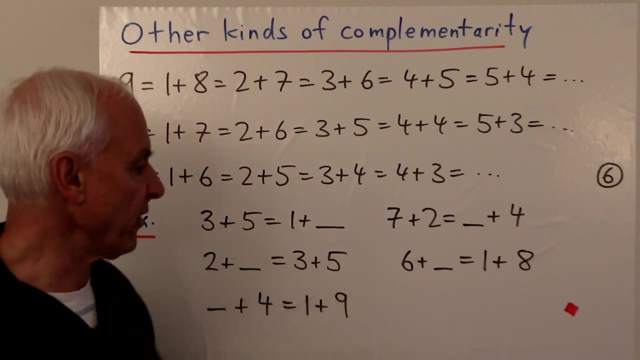 Familiar with them. if they see them as several times, they will start to get the hang of things. all right, That's what we want. So we have two plus something equals three plus five, six plus something equals one plus eight, and so on. Okay, and I think this way of writing something, where you write an equation and there's a line underneath, 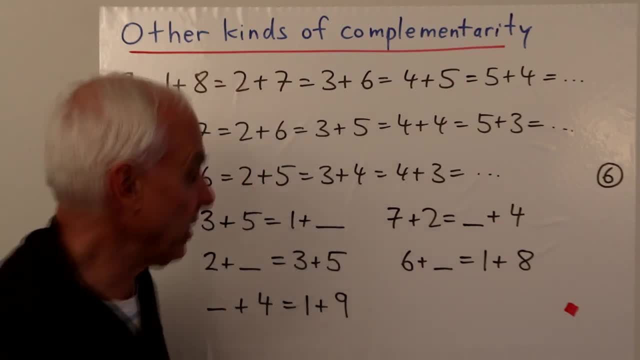 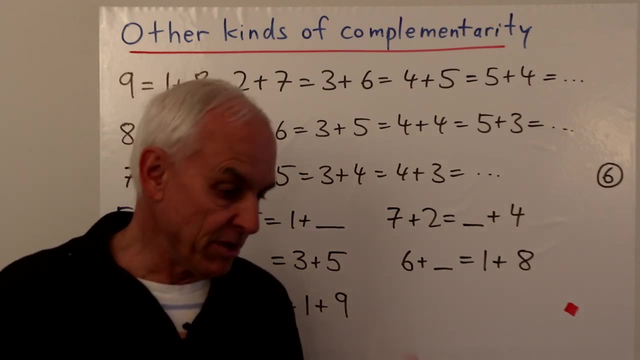 Representing a number that has to be determined is great, because the student can then just write the answer down on the question without having to repeat anything. After all, some of these students are very young. they may be Kindergarten or year one. they're able to do this kind of problem, but they may not actually be very good at actual 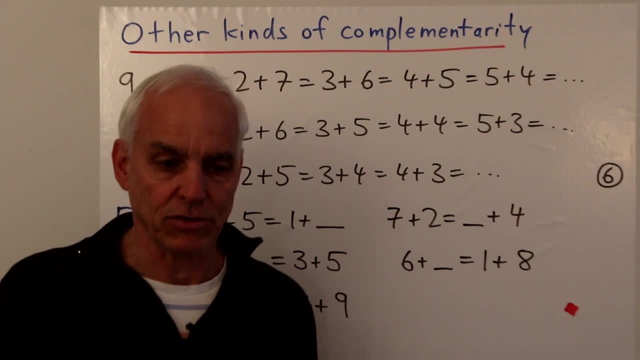 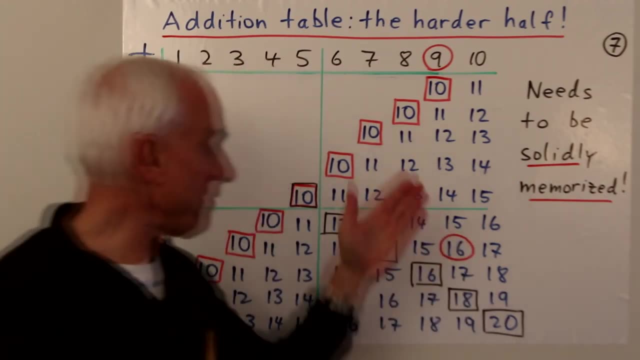 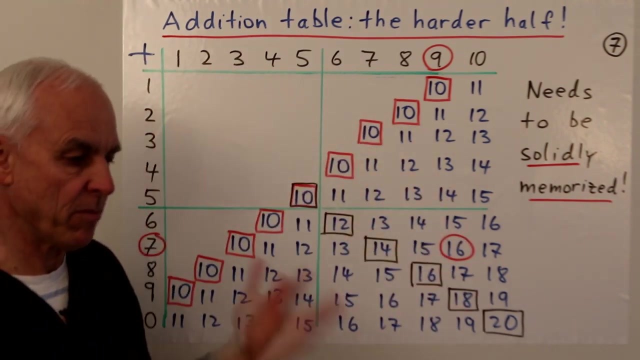 Printing or writing. okay, but hopefully they have learned how to express the natural numbers from one to ten. So after our children have learned the easier half of the addition table, now It's time to progress to the harder half, this part down here where the numbers involved are bigger. 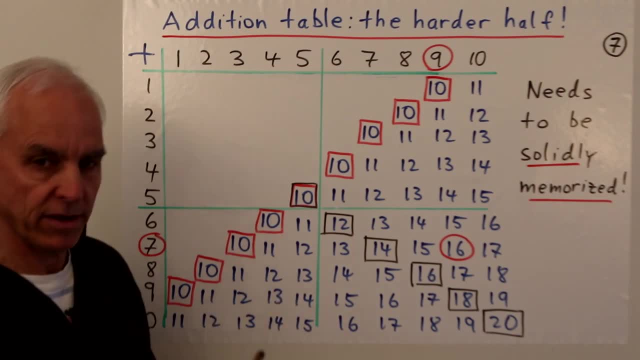 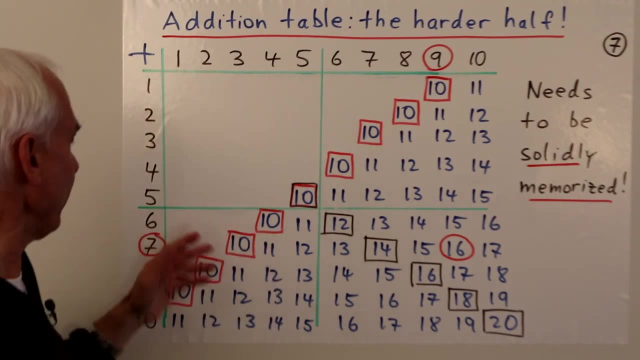 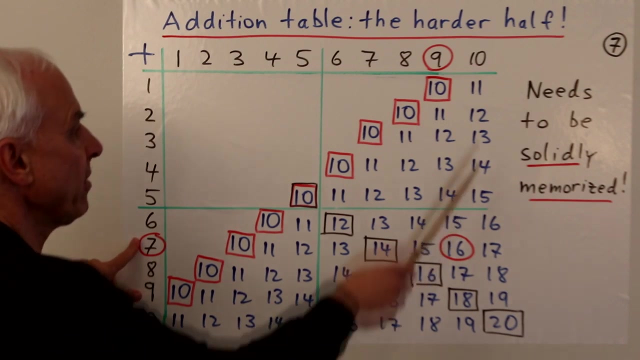 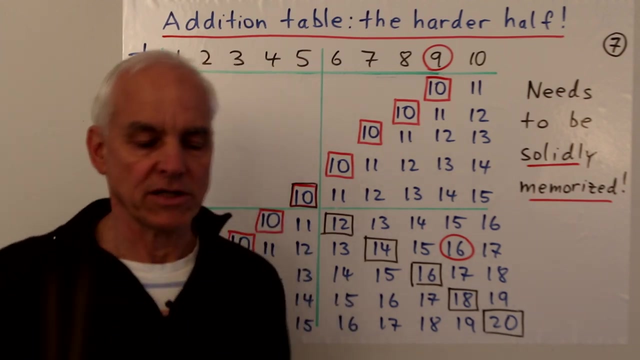 and typically in the range from ten to twenty instead of from one to ten. Okay. so They have to learn this. they have to learn that four plus eight is twelve, That five plus nine is fourteen. circle here: seven plus nine is sixteen, Okay. and you have to go through this line by line. You have to look at lots of examples, You have to illustrate things. 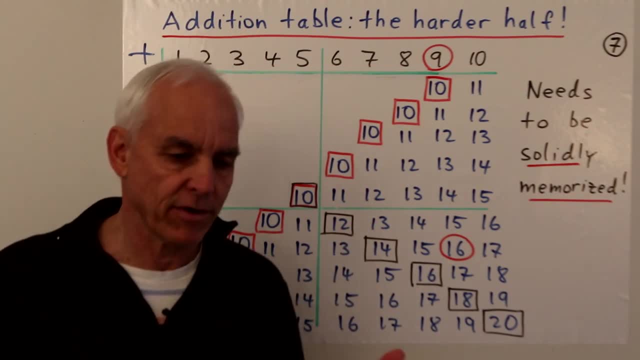 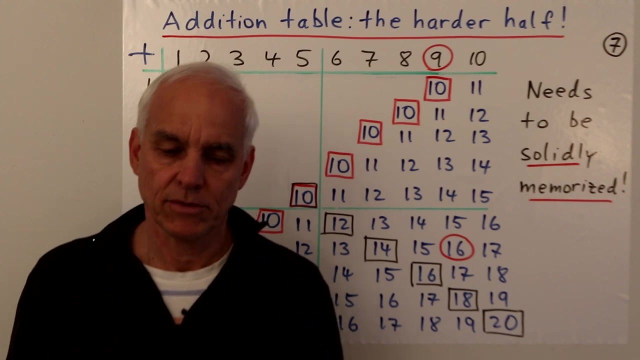 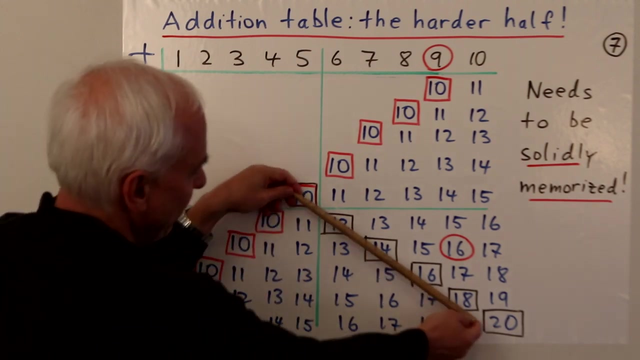 Maybe use flashcards. Whatever you know, it works, but one way or the other you want them to learn, Learn all these additions. So this, this content has to be solidly Memorized. there's various tricks for doing that. It's really not that Much, because in fact there's a kind of a reflection symmetry, right once we know what seven plus nine is. 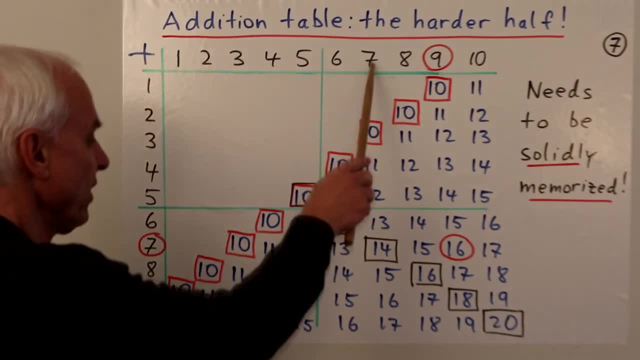 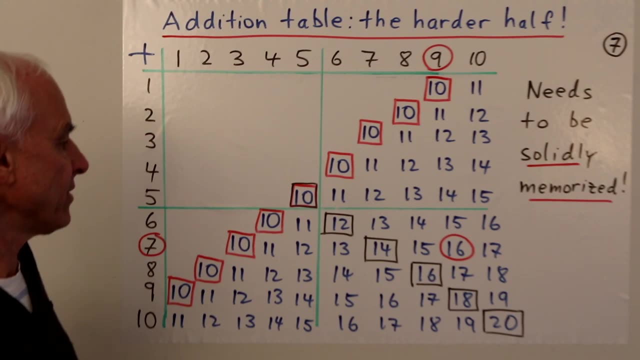 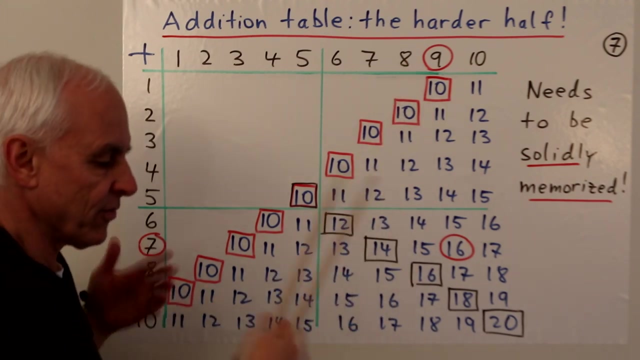 Then we also know what nine Plus seven is okay, because there's a symmetry here. so that's making the job simpler. And you know, once we know that five say seven plus nine is sixteen, well then seven plus eight is one less. You know sort of. you know we can connect the things that you do know with things that perhaps are not so solid. 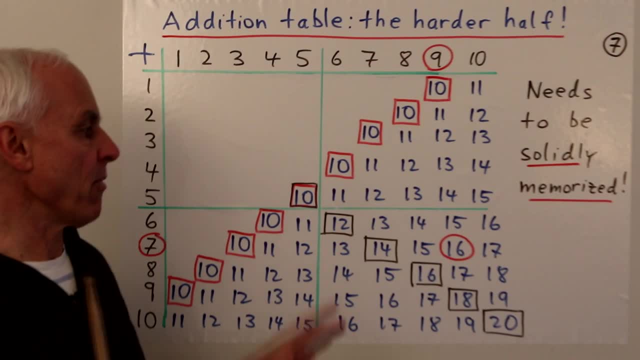 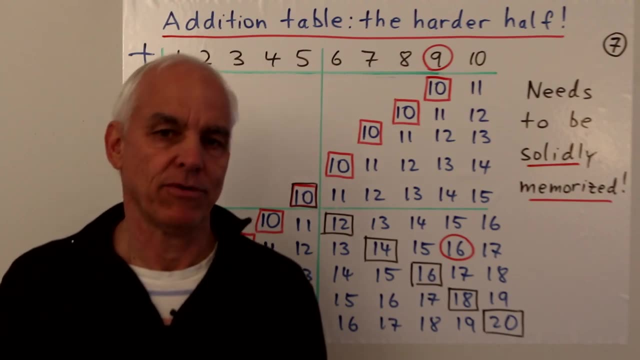 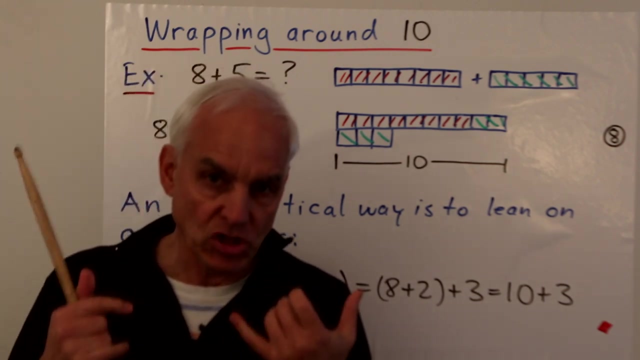 But one way or the other, Students have to become really, really familiar with this addition table, Especially this harder half of the addition table. It's crucial Now to make it easier for students to learn this. I think it's useful to have this Geometrical underpinning of what's going on, which I call wrapping around ten. 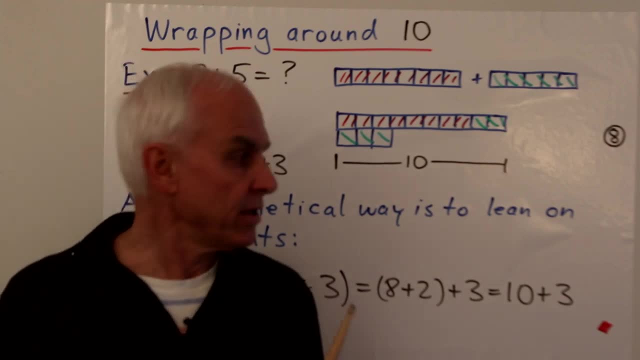 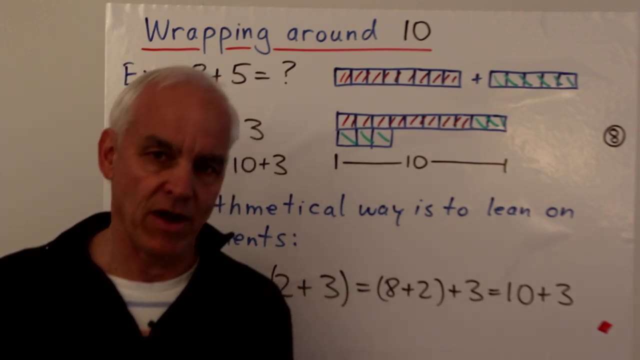 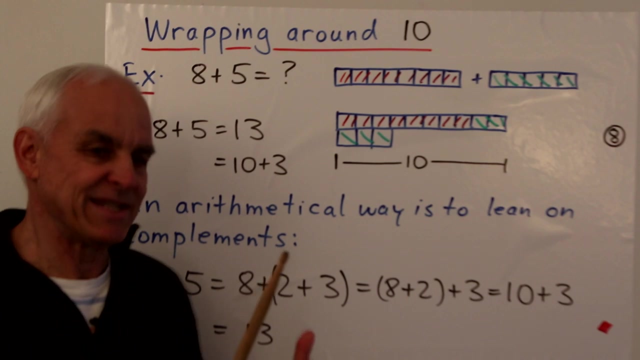 Okay. so what we're doing is we're kind of wrapping around ten. I want to illustrate What's going on here. So let's say we're interested in eight plus five. we want our student to understand What is eight plus five. Of course, eventually they'll learn that it's thirteen and then they should memorize that. but we want them, at least initially, to see that. 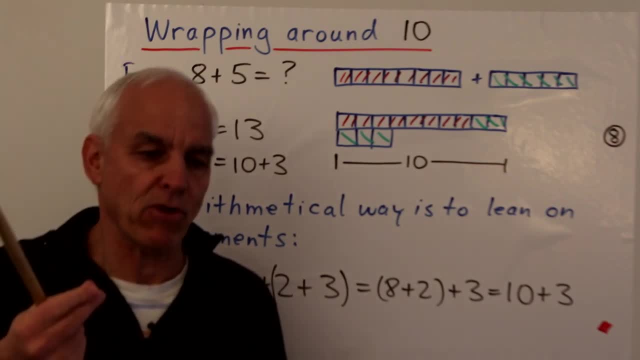 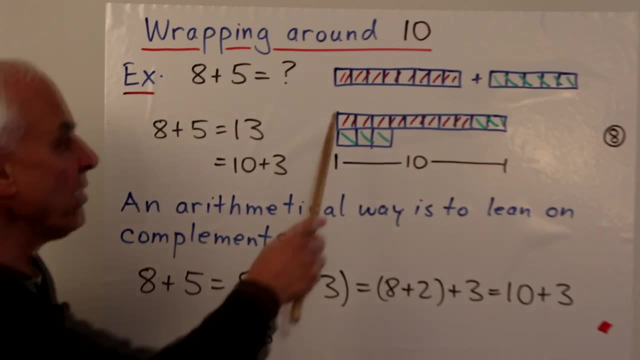 That's really true. It's not just some arbitrary thing that we're memorizing. We're actually memorizing something That makes sense. Okay, so how do we see that? Well, here is eight as a row rectangle, and here is five as a row rectangle. 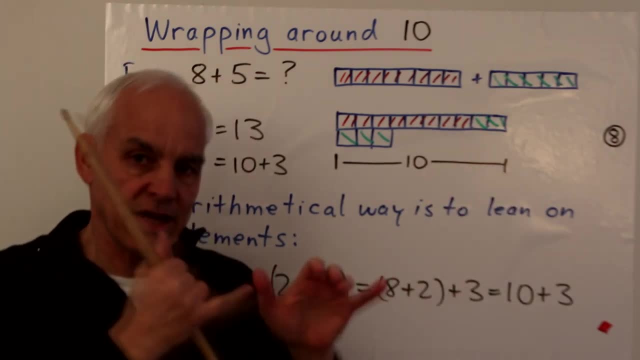 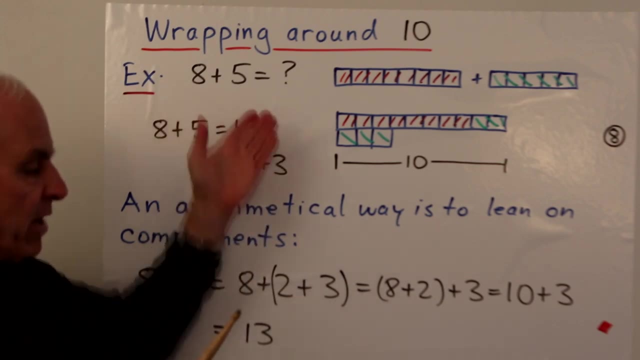 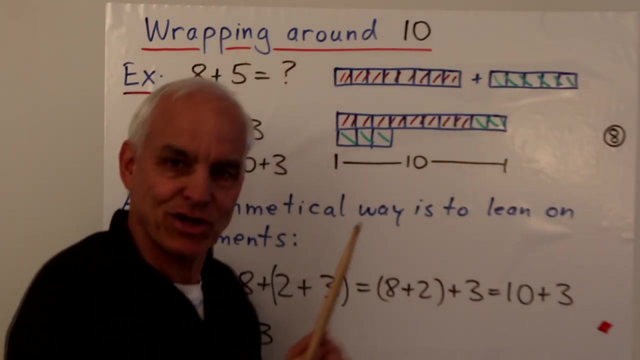 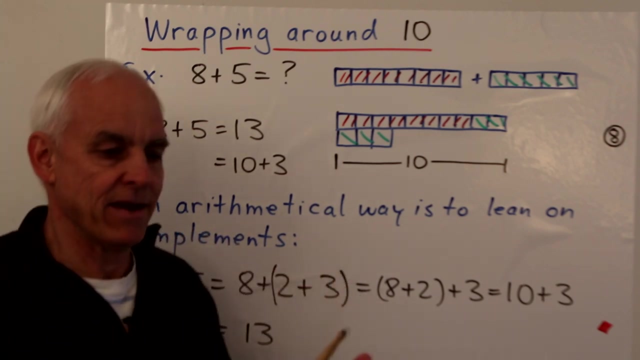 When we're adding them. what we're doing is we're putting those together to form a longer row rectangle, but with these bigger numbers that's starting to get onerous, because it's hard to identify just how big such a longish row rectangle really is. So what we do is we employ a trick or we lean on our base 10 system. 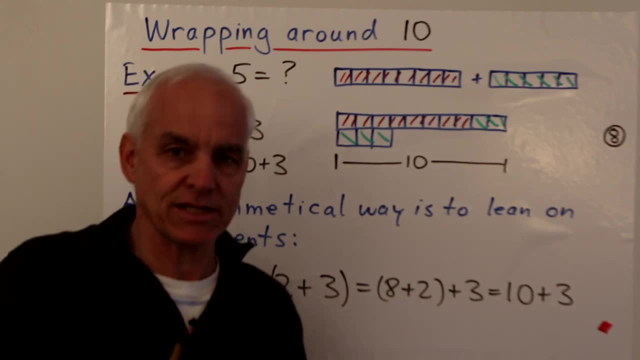 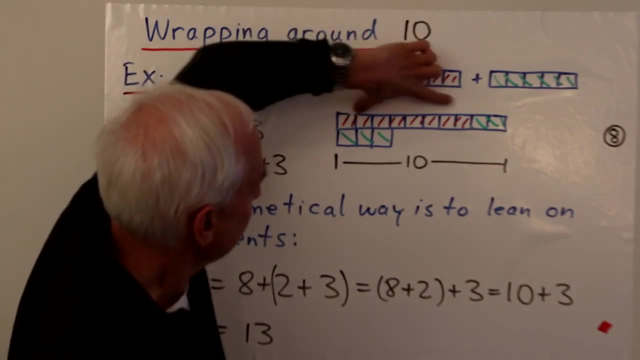 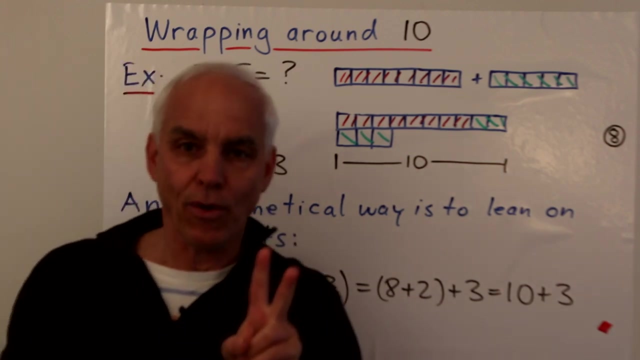 the fact that 10s are useful kind of units to separate out. So what we do is we take this 8, there's copy it again in red, that's 8, and we remember that the complement of 8 is 2.. Okay, so here's where the complementary understanding. 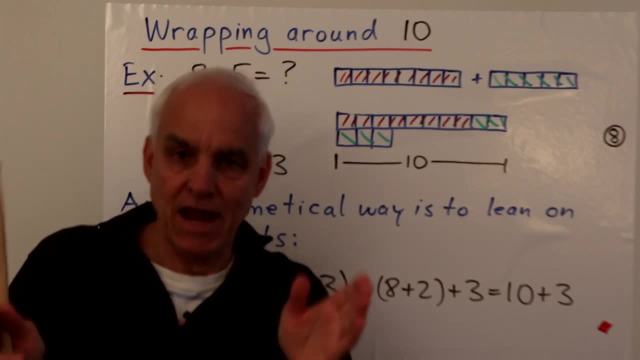 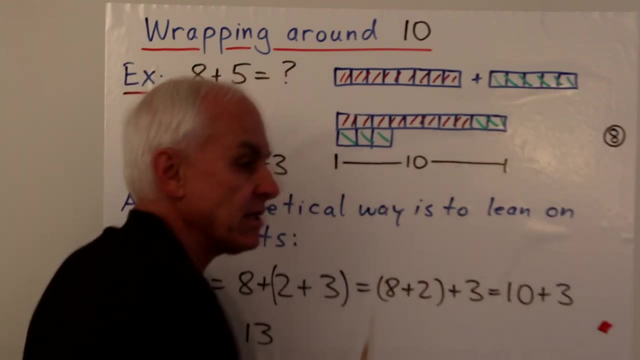 helps us. The complement of 8 is 2.. In order to get 10 from 8,, you have to add 2.. So what we're going to do in our minds is we're going to take 2 of these 5. 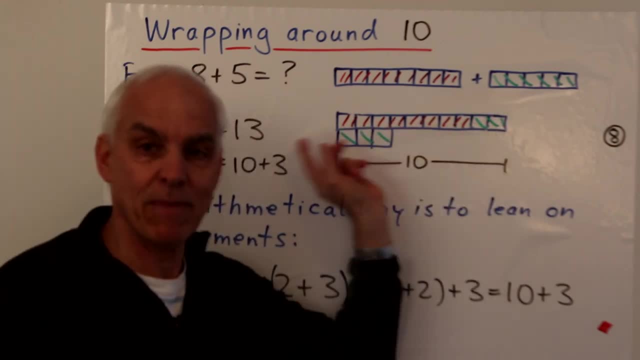 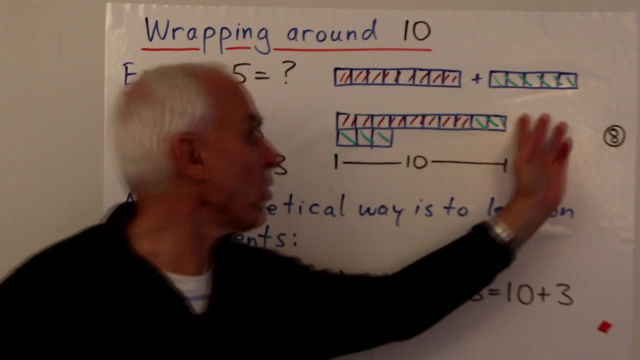 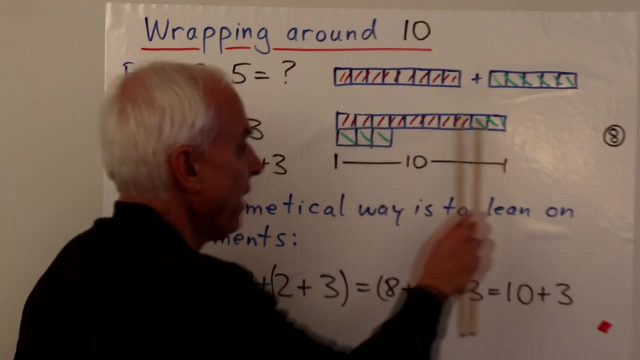 pieces and we're going to join those with our 8 to make a row of 10.. Okay, so 2 of those are going to go to the 8 to make a row of 10, and the other 3 are going to come down for a new row. Now what we see is a row of 10 and a row of. 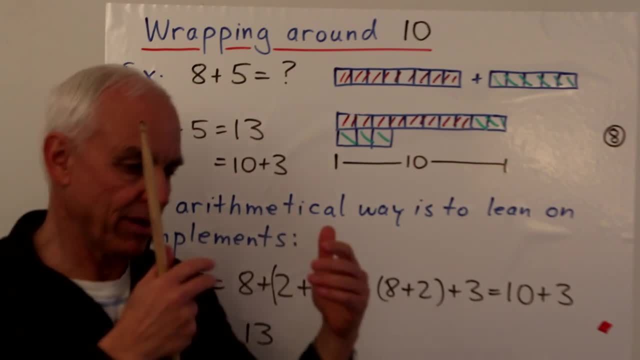 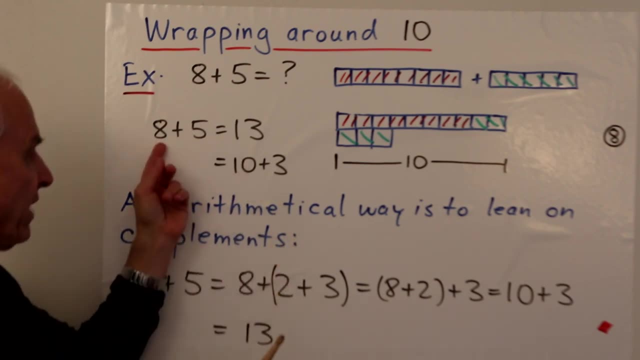 3.. That's a geometrical explanation of why 8 plus 5 is 13.. It's because we've done this intermediate step of writing it first as 10 plus 3. So complementary numbers are a useful tool to make this happen. So in some sense, what we're 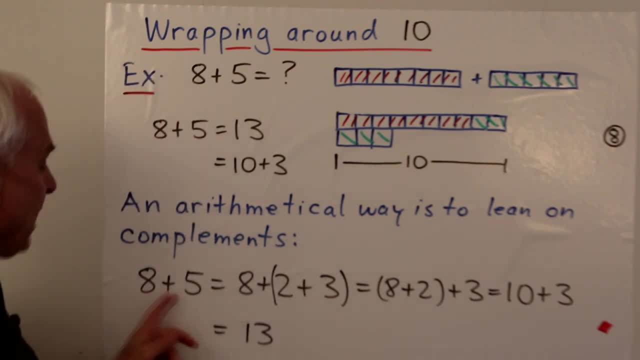 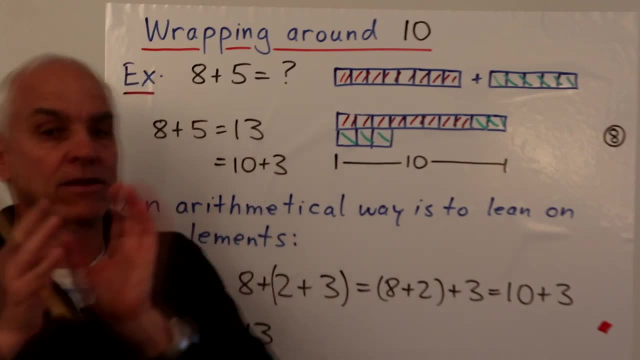 actually doing is using the associative law. What we're doing is we're saying 8 plus 5 is the same as 8 plus 2 plus 3.. We're breaking up the 5 in our minds as 2 and 3.. And we're doing that because when we rearrange that as 8 plus, 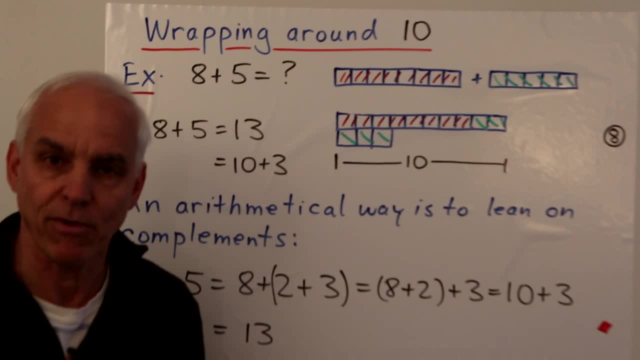 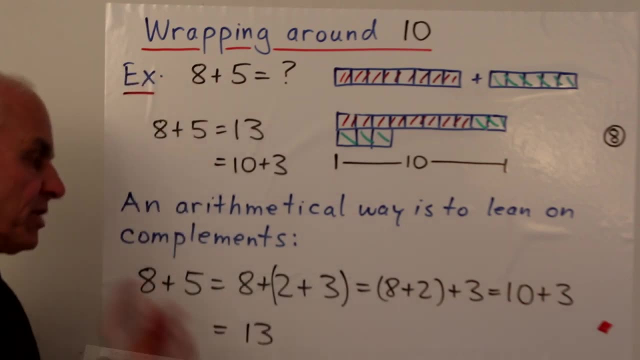 2 plus 3, these are complementary numbers. They add up to 10.. Okay, they add up to 10, so we end up with 10 plus 3, which is 13.. So this idea of going out to 10 units, 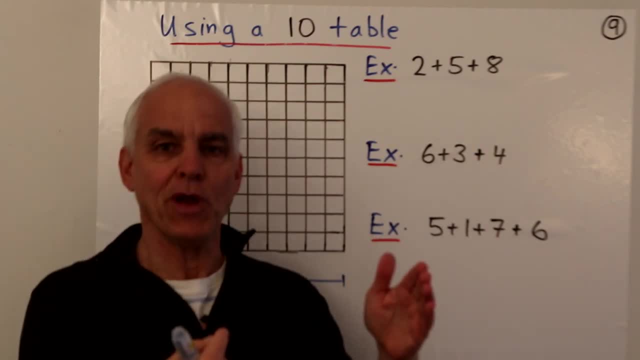 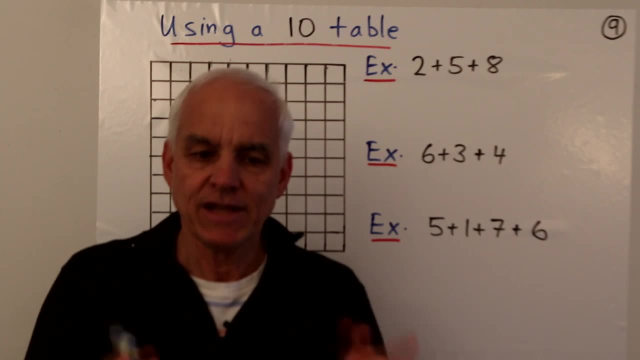 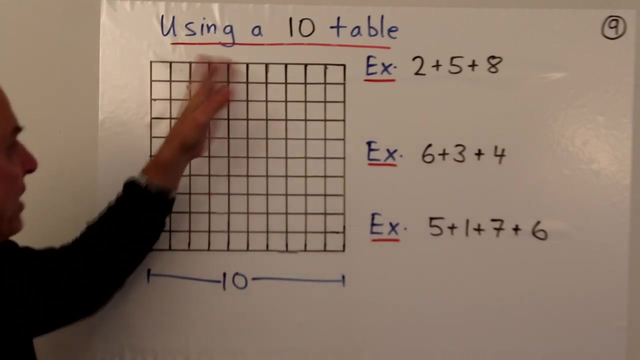 and then sort of carriage return going to the new line, is a very useful one geometrically because it allows us to visualize large numbers. So we're doing the same thing with the larger numbers, still using our row rectangle orientation. Okay, so let me show you that by introducing this thing, which I 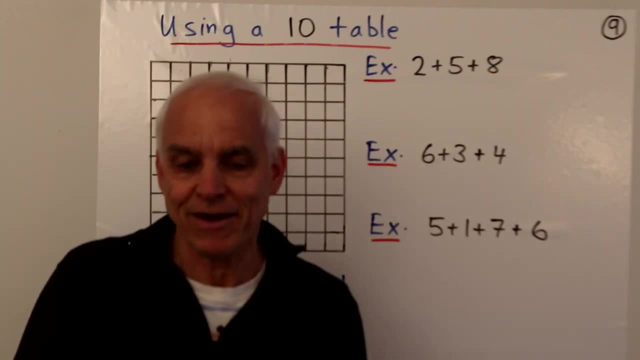 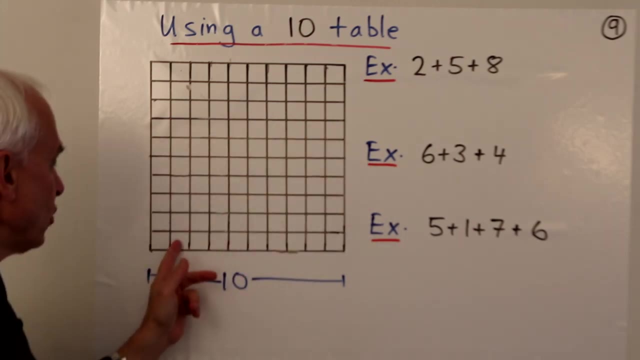 might call a 10 table. So it's a piece of graph paper. okay, like a portion of the graph paper, a column which is exactly 10 wide, 10 squares wide, 1,, 2,, 3,, 4,, 5,, 6,. 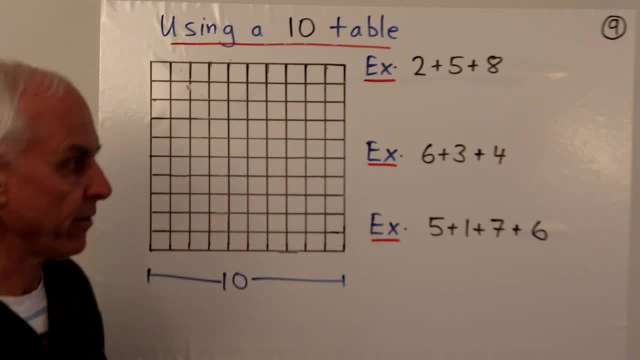 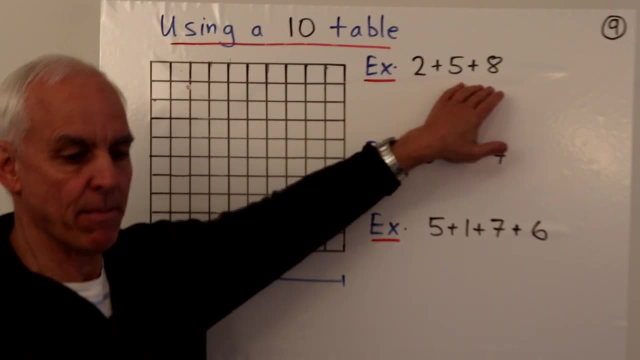 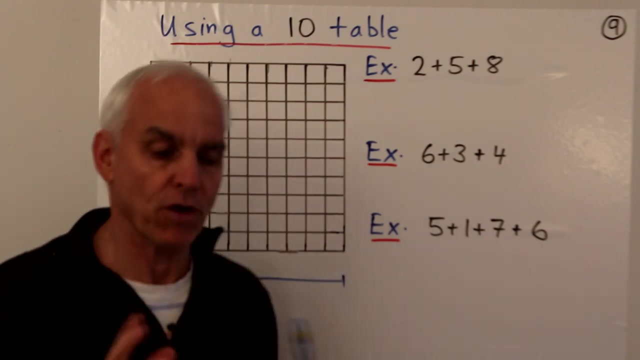 7,, 8,, 9,, 10.. Okay, and how high it is, it doesn't matter. So we're going to use this to represent what happens when we add some numbers together, including this wraparound process associated with the harder half of the addition table. So 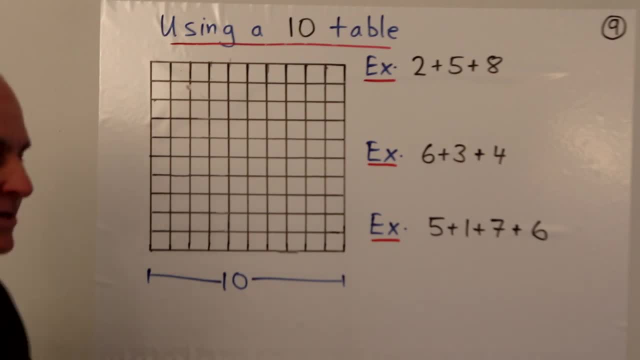 let's say we have to add 2 plus 5 plus 8.. Okay, so the 2,. there it is right. there, Okay, there's a 2.. Maybe I'll just go like that to represent that 2.. And then the. 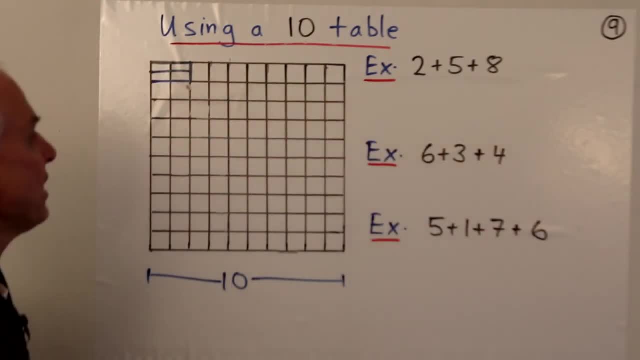 next one's 5.. I might do that in a different color to make it clearer. Okay, now we have to add a rectangle of 5.. Okay, starting there, 1,, 2,, 3,, 4,, 5.. There's a. 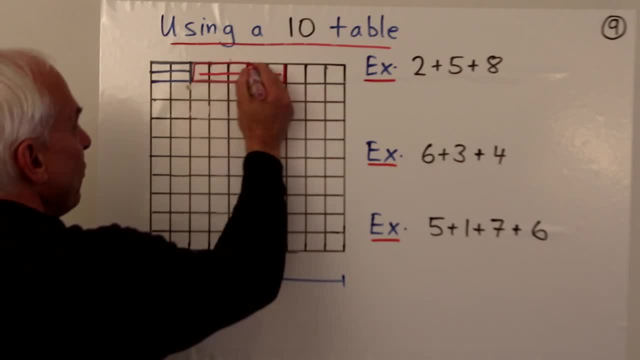 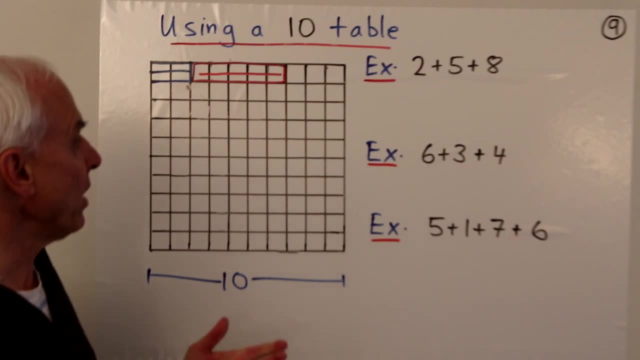 rectangle of 5.. We can actually outline it, but we're not going to keep doing that. Okay, there's a rectangle of 5. And now we have to add 8. And, geometrically, what you can see we need to do is we need to think of this 8 as kind of breaking it up. Okay, 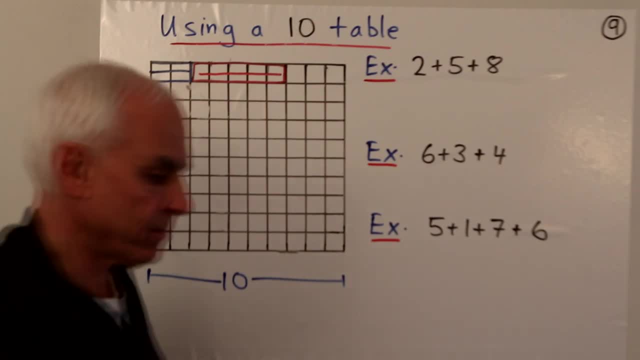 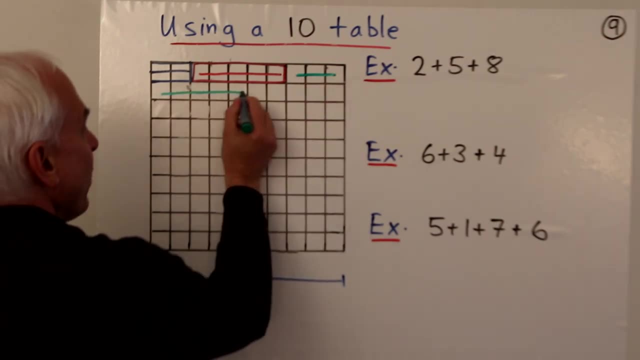 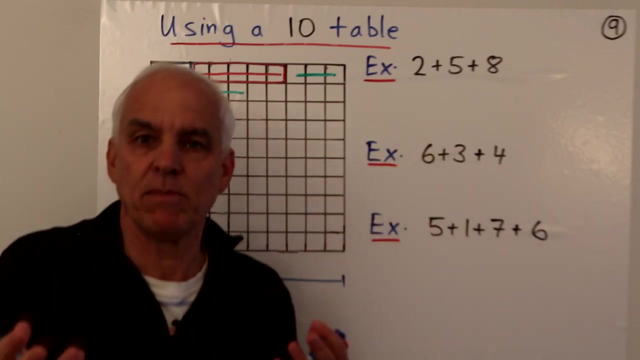 breaking it up into 3 plus something else. Maybe I'll do it in a different color So it can be 3 plus 5.. So here's where it's useful to know the complementary pairs that make up, say, something like 8.. To know that 8 is 3 plus 5.. Or maybe 2 plus 6 in another. 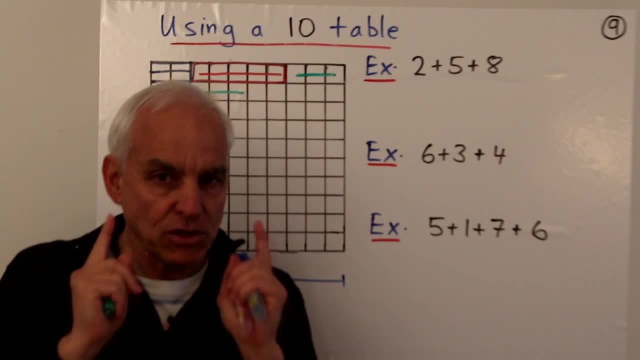 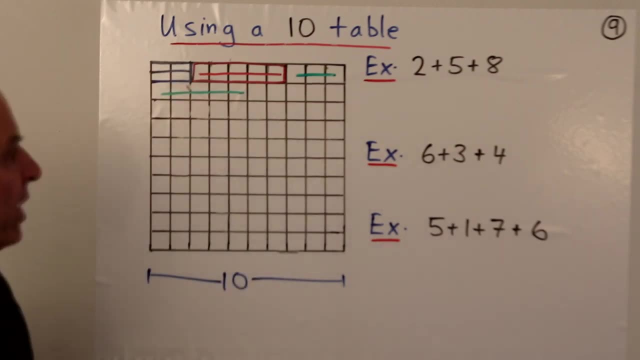 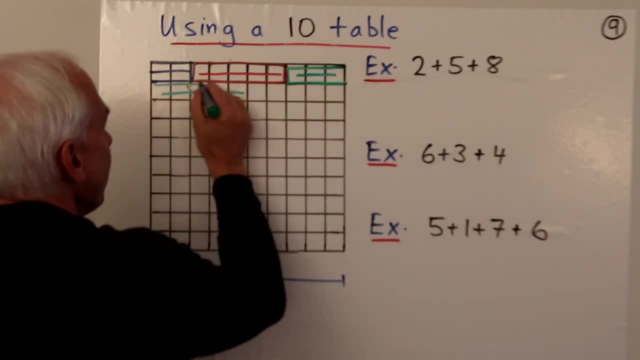 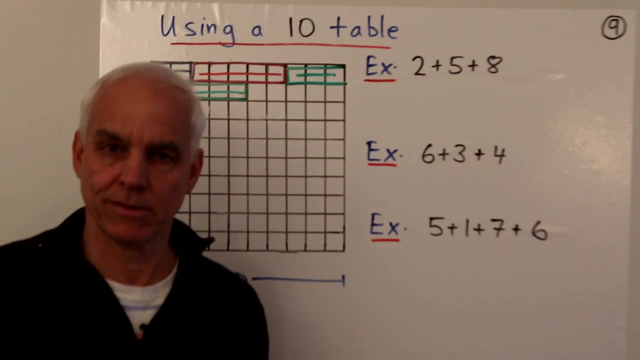 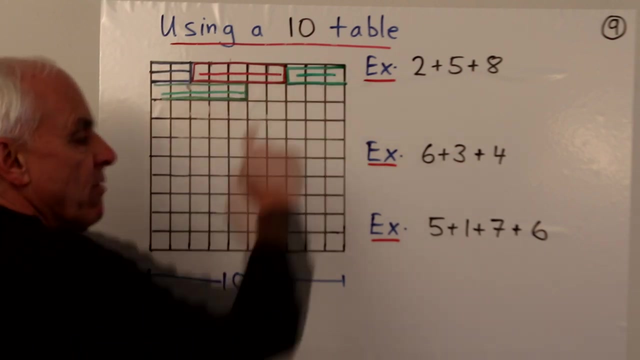 part of the rectangle of the 8.. And here is the rest of it. We've kind of broken it up and put 1 on the line that we're on, And then the rest of it in the next line, And now the result is something that's easily readable, because this is a row of 10.. So we 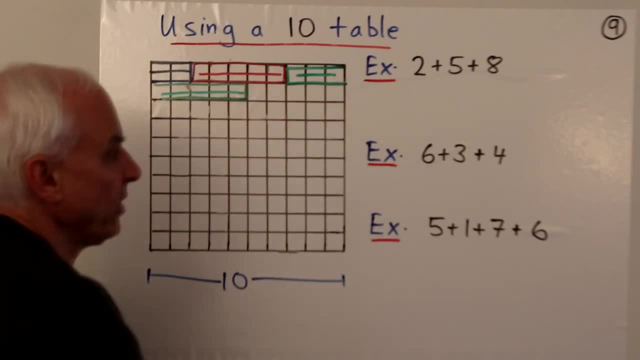 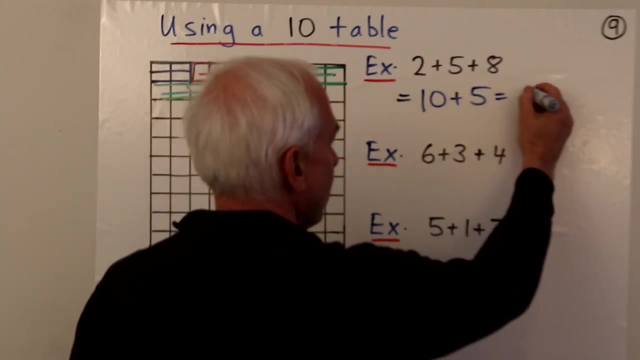 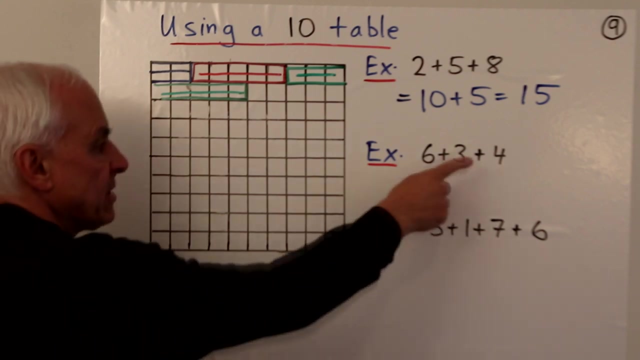 have a row of 10 with a row of 5.. So we can say that this is 10 plus 5,, which is 10 plus 5, or 15.. Let's do another example like that, Say 6 plus 3 plus 4.. Okay, I'll just. 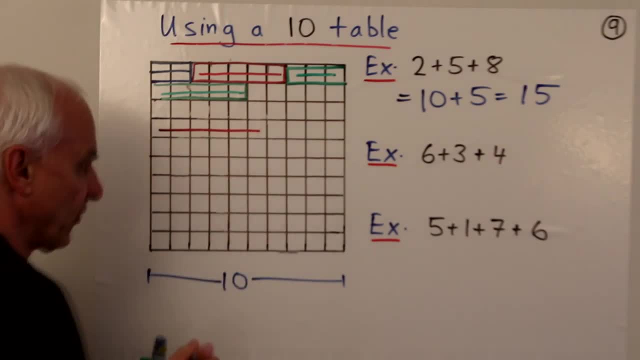 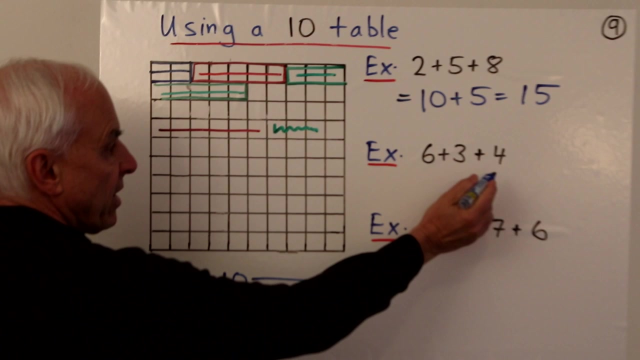 do the 6.. 1,, 2,, 3,, 4,, 5, 6.. There's the 6., All right, And then the 3.. I'll do it different. Okay, there's the 3. And now 4.. 4 is well. I need to break it up as 1 plus something. 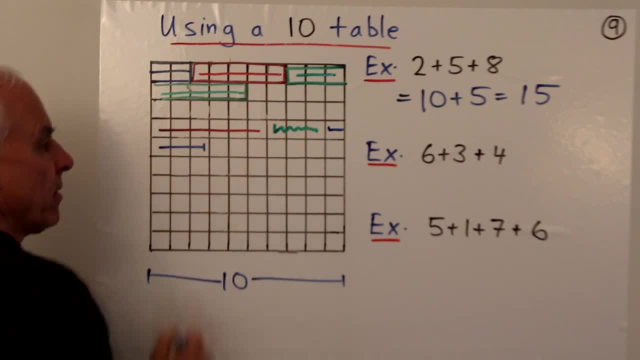 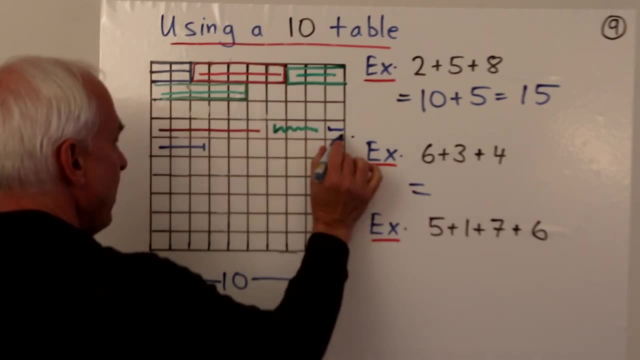 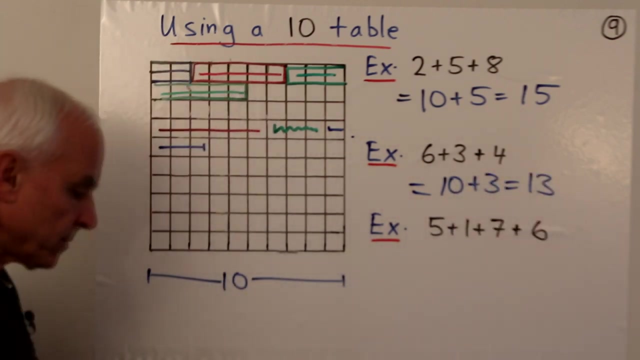 else. So it'll be 1 plus 3 more. What's the end result? The end result is that we have a 10 and a 3.. 10 plus 3, that is 13.. And let's do one more example. Let's say 5 plus 1 plus. 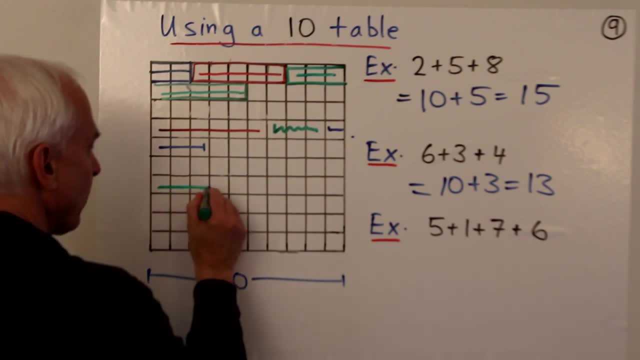 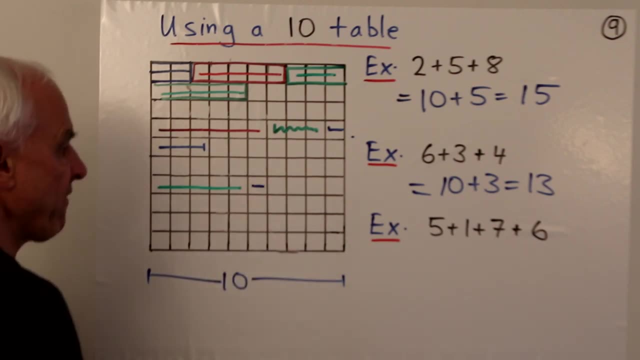 7 plus 6.. So 5, first, 1,, 2,, 3,, 4, 5.. There we go, And then 1.. Okay, there's 1.. And then 7.. Okay, so 7,. well, that's 4 of the 7. And then the complement.